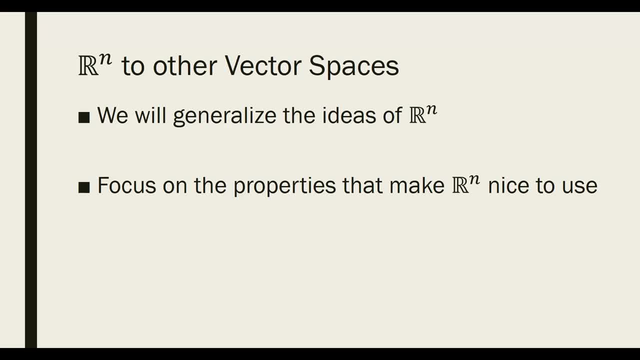 And so what the plan is for chapter 4 is we're going to take on vector spaces as a more general approach. So those ideas we found in Rn, we're going to generalize those ideas and we're going to focus primarily in this section on some properties that make Rn nice. 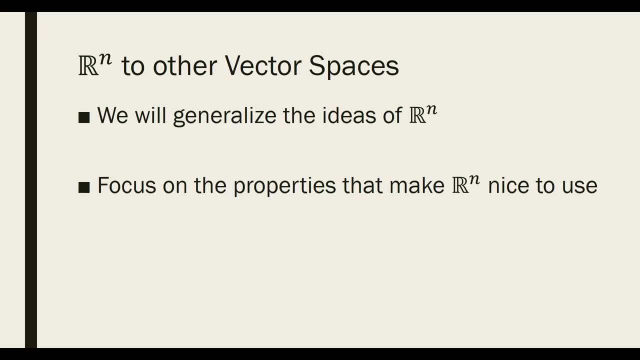 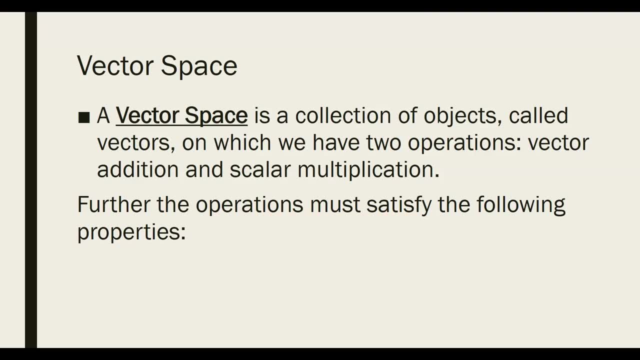 and generalize out to to other other um spaces. So let's talk about what a vector space actually is. A vector space is any collection of objects called vectors on which we have two operations, which we call vector addition and scalar multiplication. 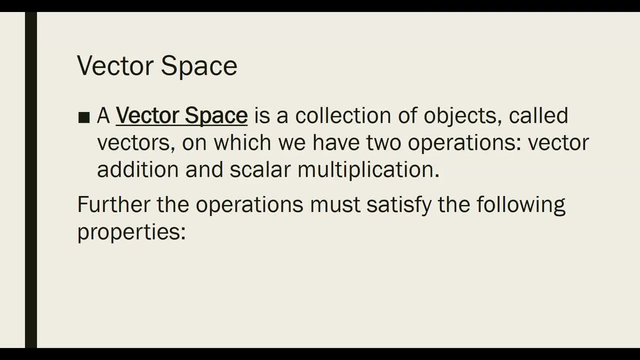 And in order to be a vector space, those operations, along with the vectors, have to satisfy some properties. Okay, So all we need is something called vectors, and those vectors can be sort of any mathematical objects we can think of, along with two operations. 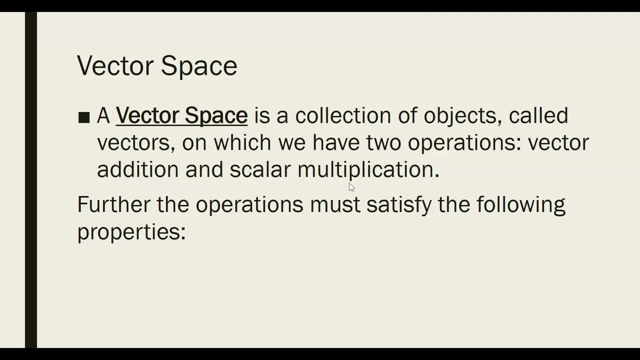 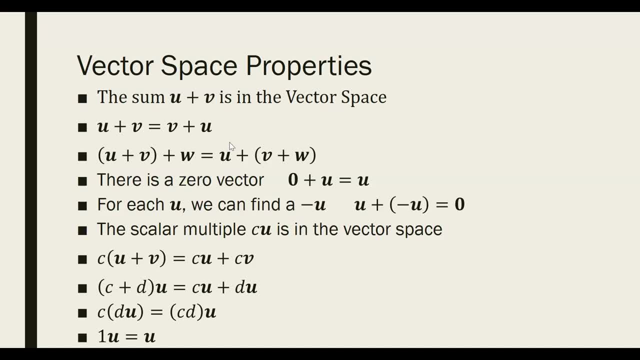 uh, vector addition and scalar multiplication- And they have to have the following properties. Specifically, if you look the sum of any two vectors from the vector space, the sum also has to be in the vector space. So this means it's. 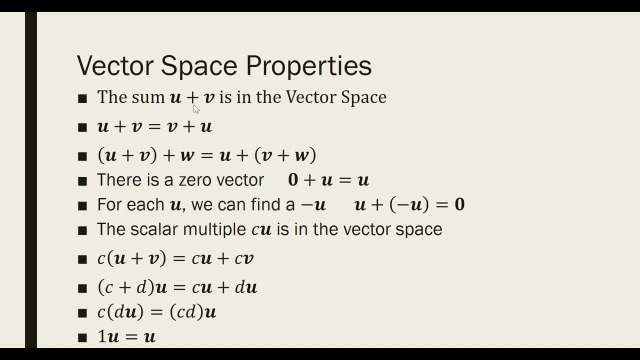 closed under addition. Alright, So if you start with two vectors, add them up. the sum also has to be in there. The vector addition has to commute. The vector addition has to be associative. We have to have a zero vector in order to have a vector space. 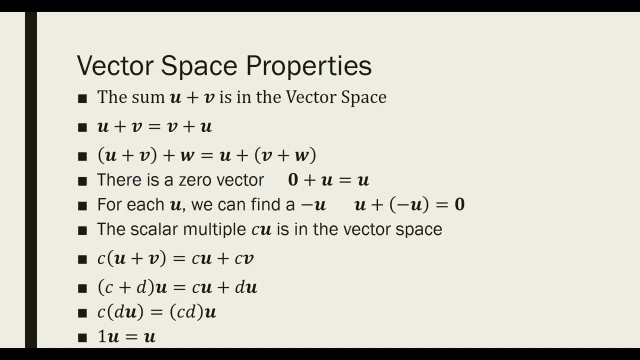 The vector where you add it to anything, any other vector, and it doesn't change Along with the zero vector. if I have a single vector u, you can always find a negative u so that they add to the zero vector. So 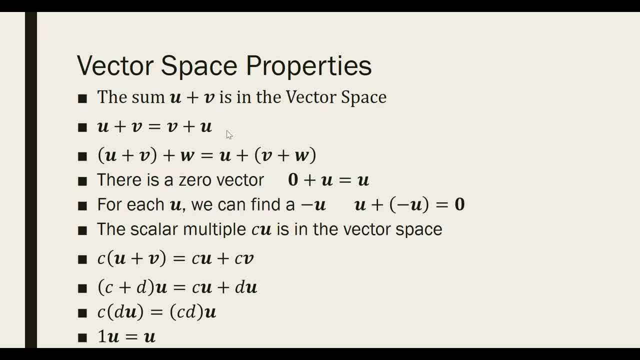 all of these are properties of addition. Closed under addition, commutative, associative, has a zero vector and you can find opposites, Alright, Additive opposites. So all of those are the properties of addition that a vector space needs to have. 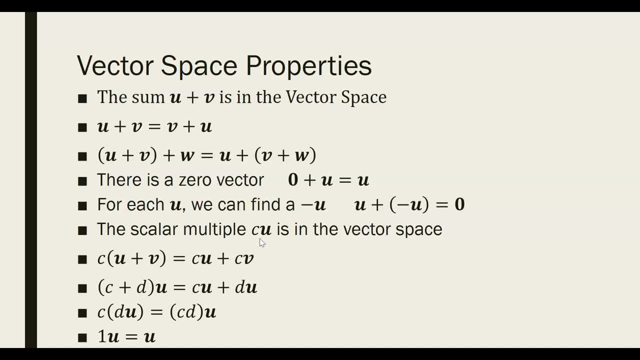 The other properties have to do with the scalar multiplication. So, first off, scalar multiplication is going to be closed. if you multiply a scalar times a vector, That is going to also be in the vector space. If I take a scalar times, two vectors added together. 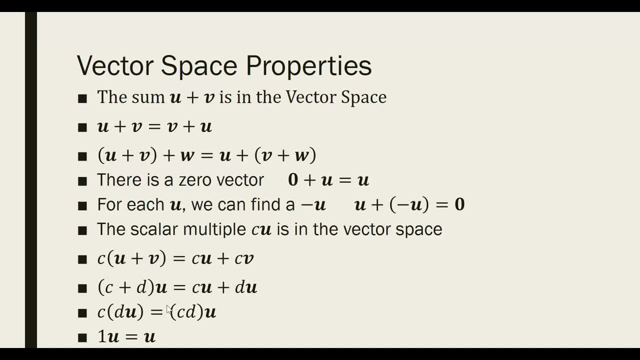 that scalar has to distribute. Also, vectors would have to distribute over scalar addition. And then scalar multiplication is associative. Also, if you multiply the number one by a vector, you're going to get no change. So all of these properties have to be. 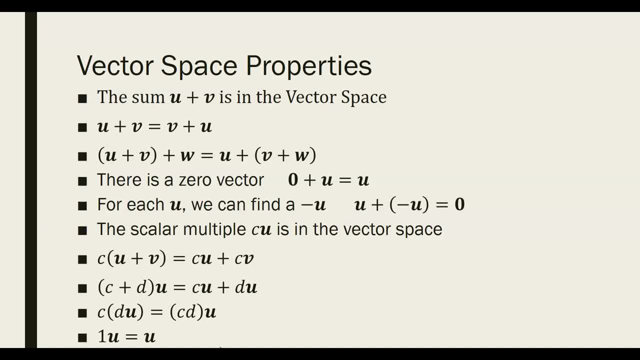 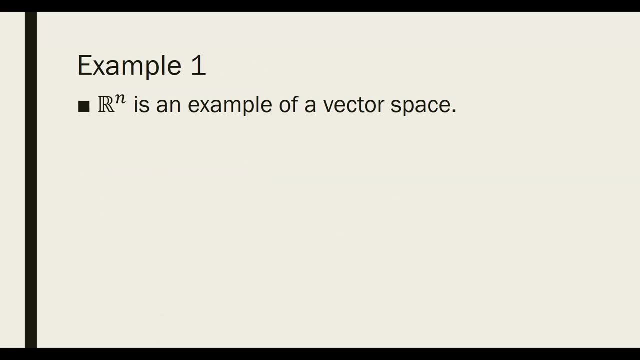 satisfied in order for our collection of vectors to actually be a vector space. And obviously the space that we've been dealing with all in chapters two and three Rn is one example of a vector space, If you think about two vectors. 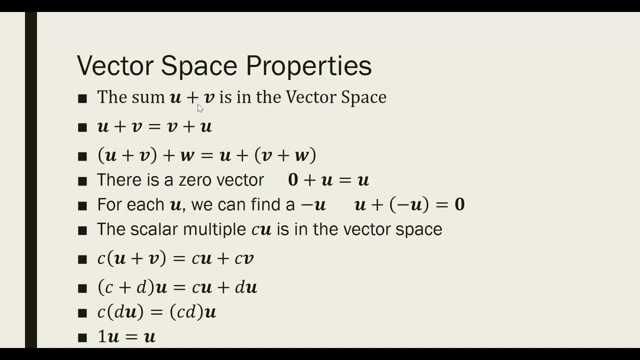 if you add two vectors that have, um, let's say, three entries, then their sum is also going to have three entries If they're real numbers. um vector addition of Rn commutes. Vector addition is associative. There is a zero vector. 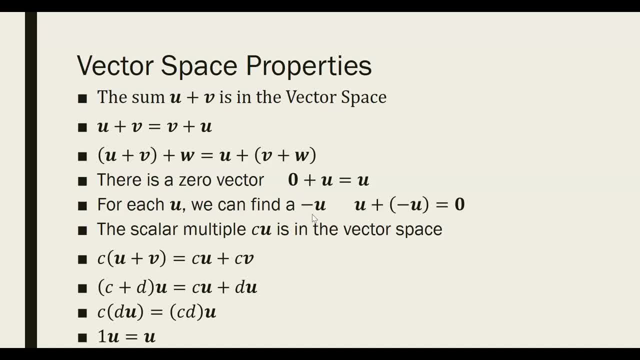 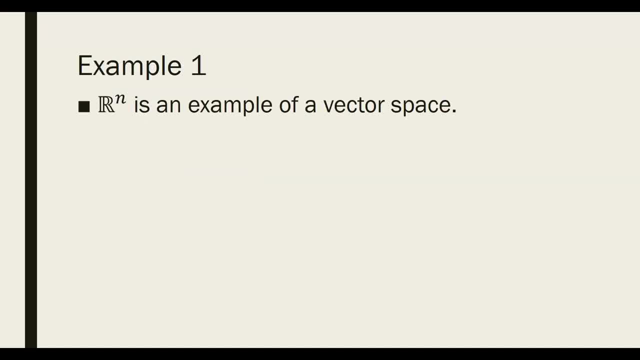 That's the Rn. with all zeros, You can always find negatives, Scalar multiplication is fine, and so on and so forth. So Rn is the example of a vector space that we've been working with before. So Rn is in and of itself a vector. 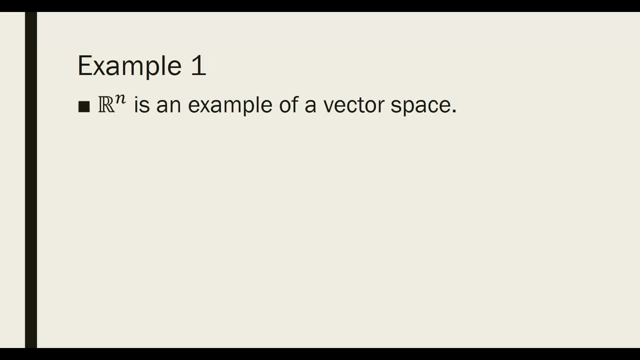 space and that's kind of what motivated, or what motivates, the idea of vector spaces. But Rn is not the only vector space. For instance, all polynomials of degree, let's say three or less, with real number coefficients. 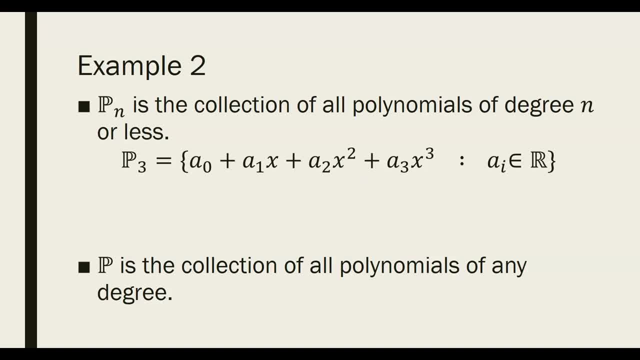 is a vector space. If you add two polynomials of degree three or less, you're going to get a polynomial of degree three or less. If you take a polynomial and you multiply it by a scalar, you just multiply each term, so you're going to end up. 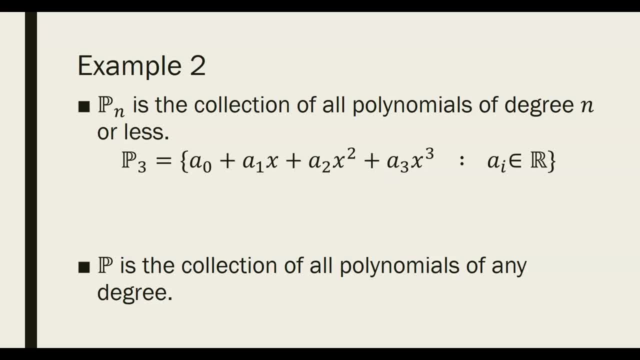 with another polynomial And the notation here: P sub n. that is the reflection of all polynomials of a degree n or less. So P sub three is the polynomials of degree four, excuse me, degree three or less. Alright, where all of our coefficients? 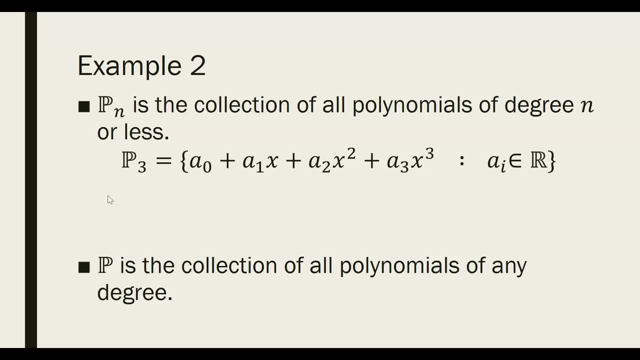 are real numbers. If you want to go infinite polynomials or if you want to go all polynomials, no matter what the degree. so P sub three, we stop at degree three. we can't get an x to the fourth, for instance. 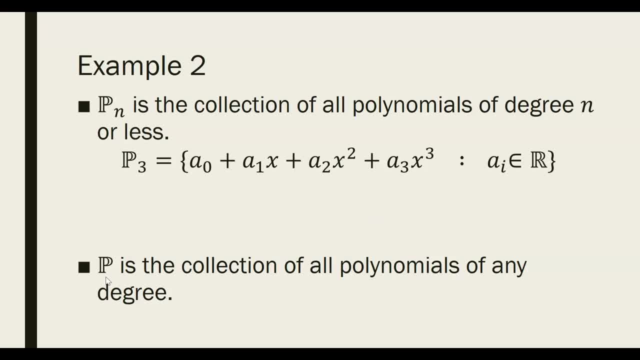 if you wanted to be polynomials of any degree, we just call that P, without a subscript, And that is also a vector space. If you think about it, you add two polynomials. it's going to be a polynomial If you take a scalar. 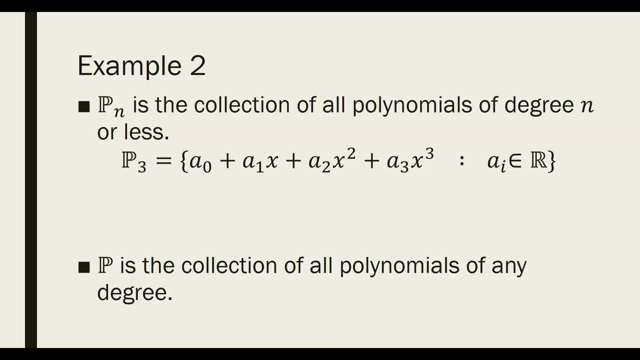 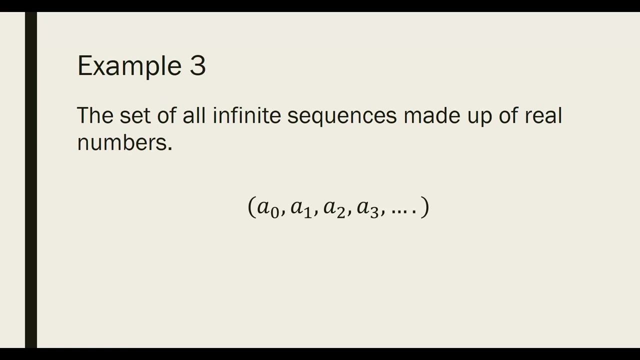 multiple of a polynomial, it's still going to be a polynomial, Alright. so polynomials of degree, any degree, the collection of all polynomials of any degree or less, is going to be a vector space. Another example of vector space is all infinite. 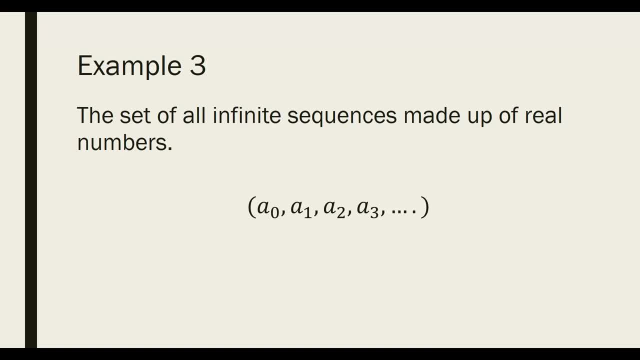 sequences made up of real numbers. So what we could do, one way to think of it, is: if we have an infinite sequence of numbers, you can think of it as the numbers themselves. you could also think of it as sort of an infinite vector. 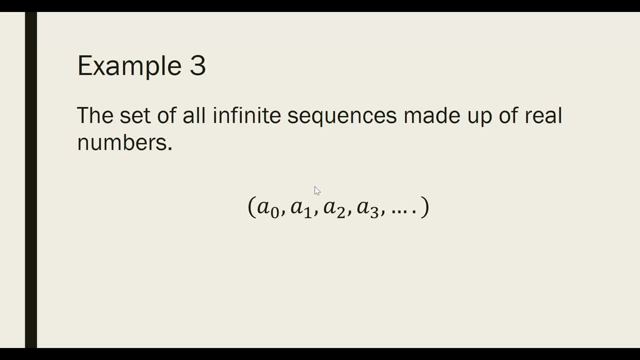 okay that we've oriented horizontally rather than vertically, So we have infinitely many entries, but the collection of all infinite sequences where entries are real numbers would in fact be a vector space. Here's another example of a vector space: functions that are defined on a set of. 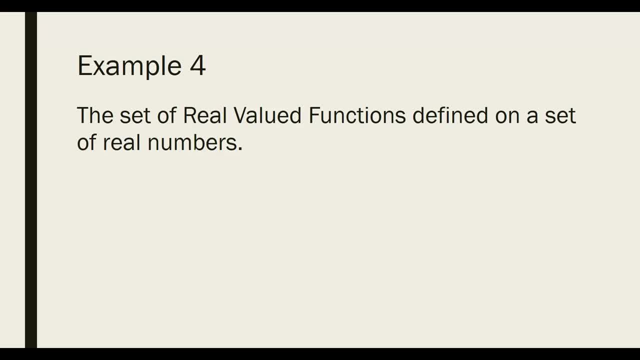 real numbers. So maybe I say all functions which are defined on the interval from 0 to 2.. So all real valued functions that are defined, you know, on a closed interval from 0 to 2, or something like this, or maybe it's all real. 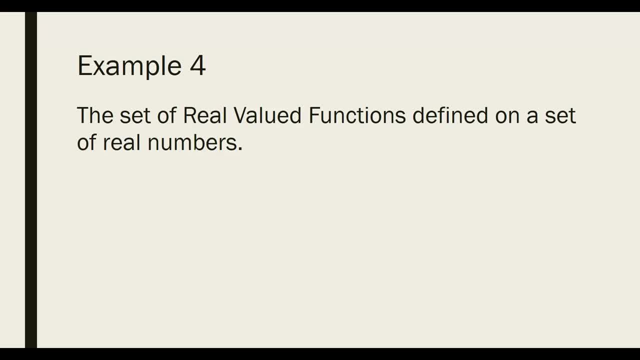 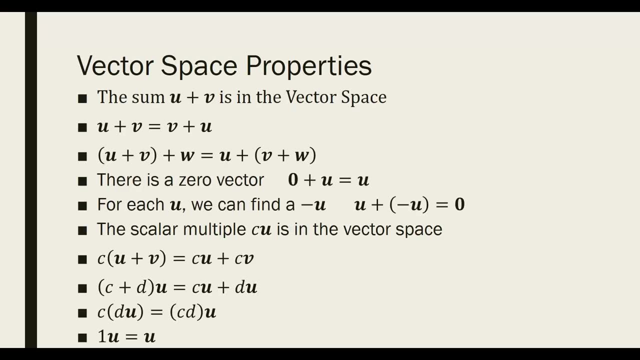 functions, real valued functions, defined on the set, on the entire set of real numbers. That would also be a vector space. So if I collect real valued functions, they are a vector space- And think about what the properties would be. Real valued function. 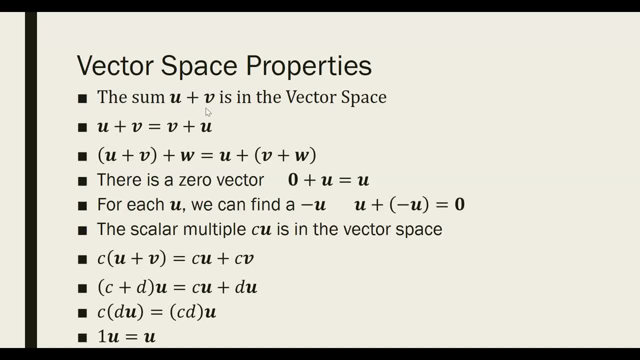 plus a real valued function is going to be a different real valued function. If I add two different real valued functions, the order in which I add them are going to matter. There is a zero vector, that's f of x equals 0.. Take f of x equals. 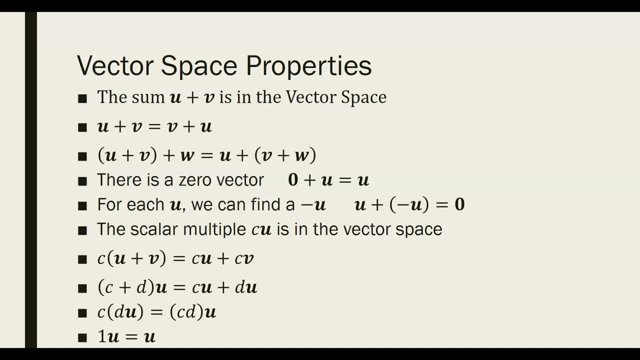 0 plus anything f of x equals 0, if you add that to anything any other function, you get back the function itself. You can negate any function you want. you can multiply any function you want by a scalar When you add. 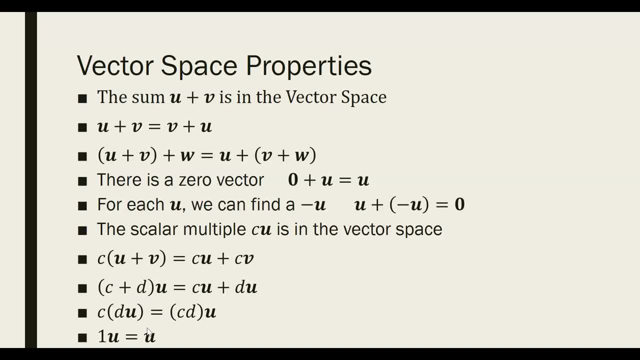 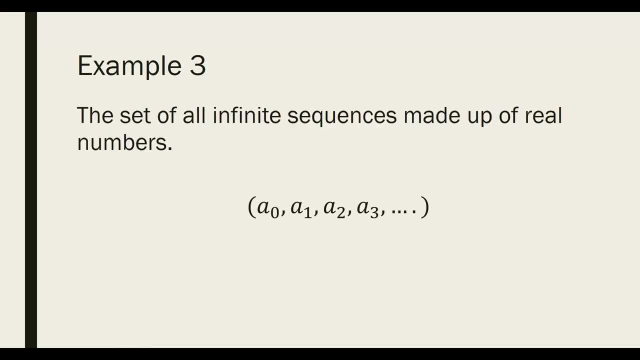 functions you can distribute with scalars, and if you take the number 1 and you multiply a function, you still get that function back. So the set of real valued functions on a set are in fact or do in fact. 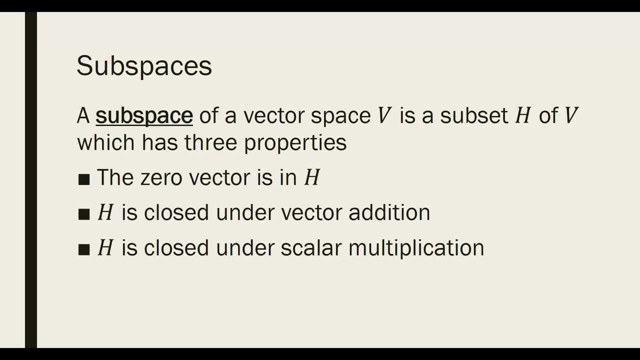 form a vector space. So vector spaces are all over and it's actually a very broad concept. We see real valued functions, we see polynomials, we see polynomials of degree 3 or less, we see infinite sequences. So all of those are. 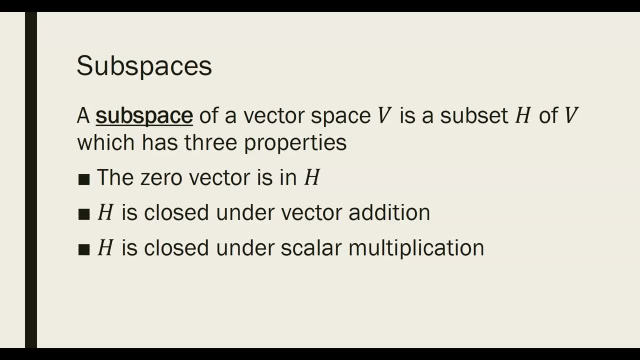 vector spaces along with Rn, And when we dealt earlier in chapter 2 with vector spaces, one of the first things we looked at were subspaces of the vector space And, just like in chapter 2, we looked at subspaces of Rn. 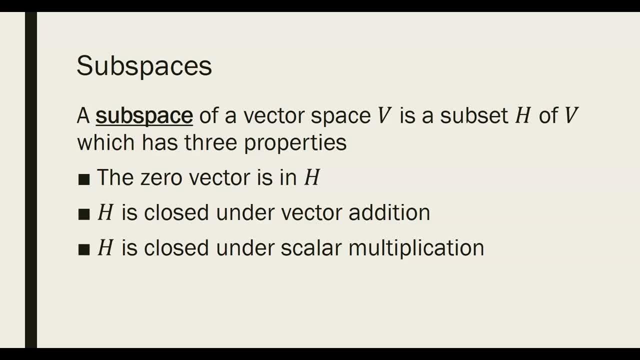 now we can generalize subspaces to be any set which is a subset of a vector, space V, such that three properties hold. The first property is that the zero vector has to be in my set, so that my subspace has to contain the zero vector. 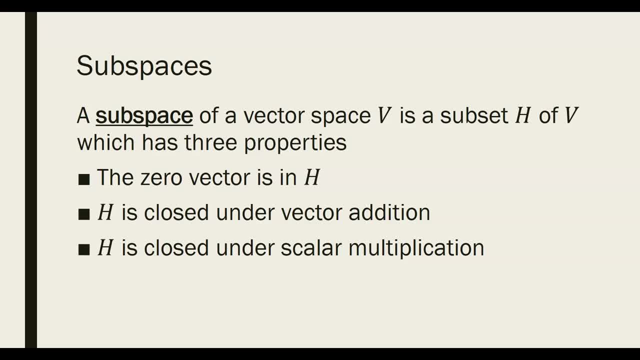 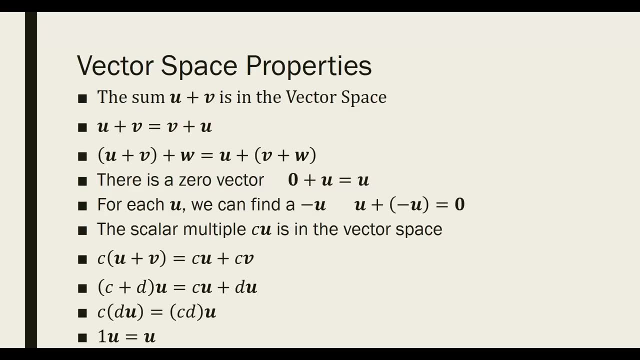 The second property is that my set is closed under vector addition. And then the third property is that my set is closed under scalar multiplication. Now one thing: if I scroll back to what vector spaces were, notice that to be vectors in a space we have to have 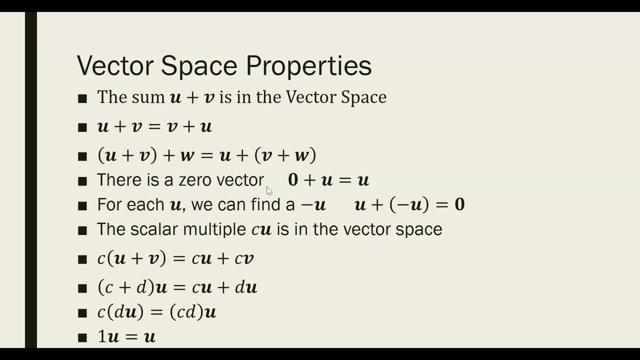 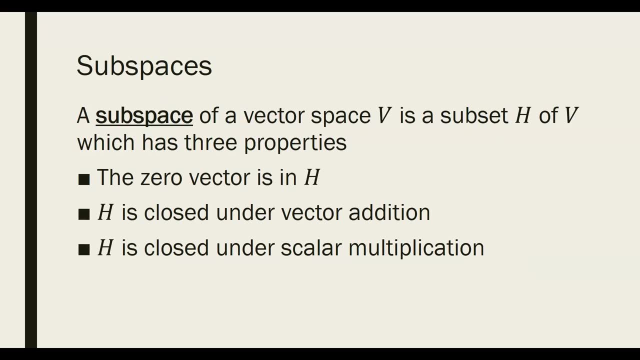 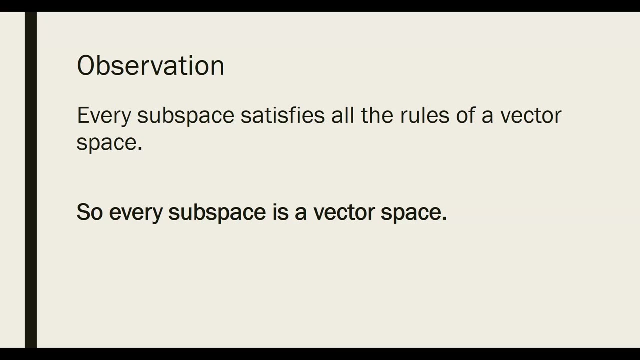 commutativity, we have to have associativity, we have to have negatives, we have to have scalar distribution, all that kind of good stuff. So what I want to say is that a subspace is, in fact, a vector space itself. Alright, 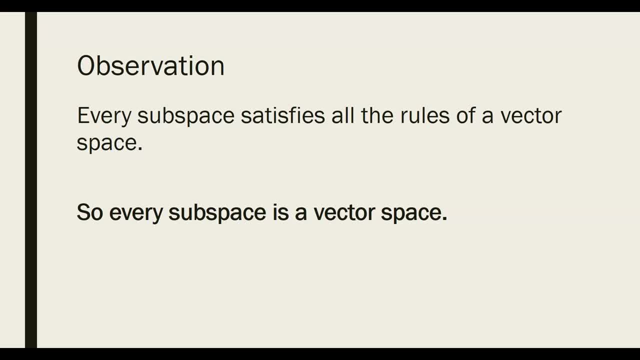 As long as your subspace satisfies those three properties- I mean, as long as our set satisfies the three properties- to be a subspace, you're going to sort of get the other properties for free, because we know our subspace is a collection of vectors. 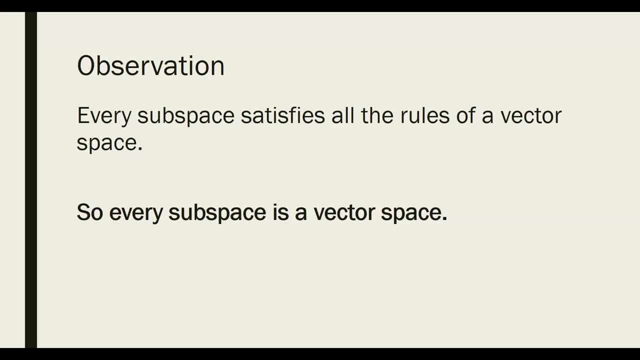 Alright. And all vectors have to be commutative. All vectors have to have commutative addition. All vectors have to have addition which is associative. All vectors have to have nice scalar multiplication properties. So as long as we can show that the zero vector 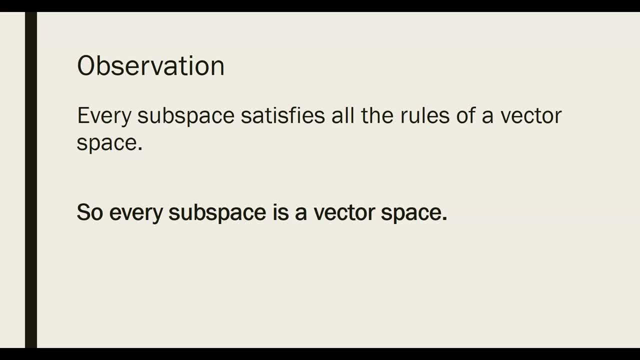 is in our subspace, that. let me repeat that, as long as we can show that the zero vector is in our set, that the set is closed under addition and the set is closed under scalar multiplication, then we know that we get a subspace. 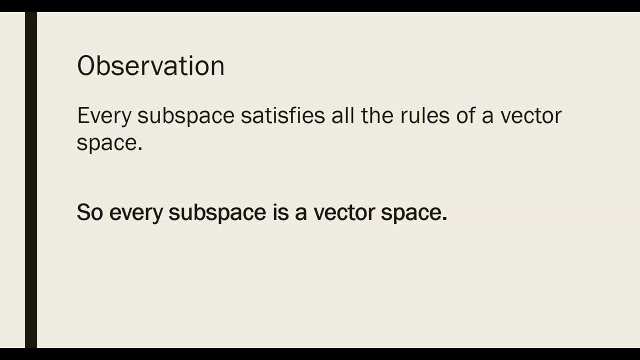 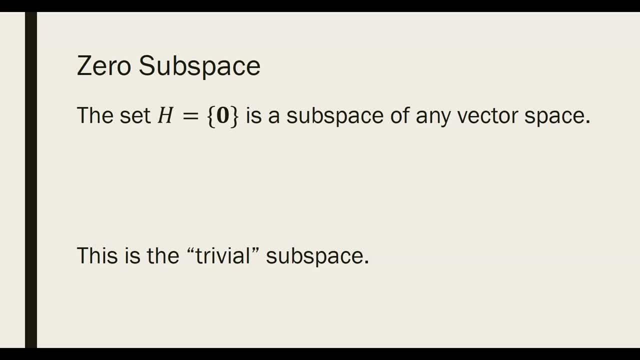 and, moreover, we know that that subspace is in fact, a vector space itself. Now, we saw this earlier in Rn, but I wanted to put it out there again: The set containing only the zero vector is a subspace of any vector space. 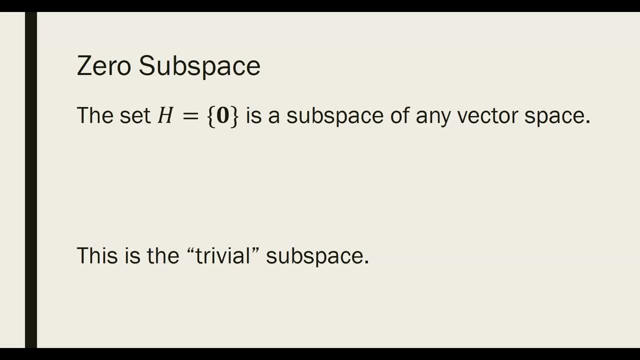 Remember, any vector space has a zero vector. so polynomials of degree three and less, functions defined from on zero to two, those types of things, all of them will have a zero vector. And if we let h be the set containing only the zero vector, 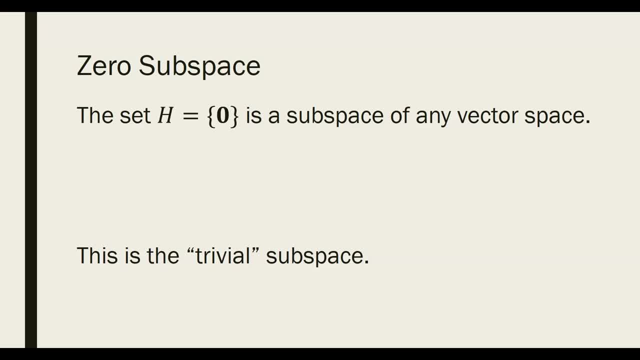 then this is a subspace called the trivial subspace. Alright, trivial subspace is the set containing the zero vector. So what we're going to do is we're going to check the three properties of subspaces for a few different collections of vectors and see if they are. 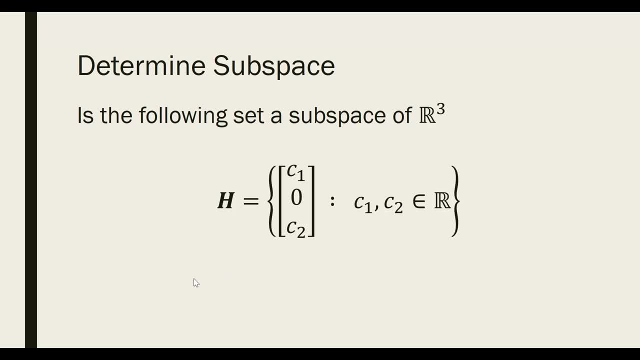 in fact subspaces. So I want you to push pause on the video and check that. check if the following set is a subspace of r3.. Okay, This is something we did before, so hopefully it won't take you too long. But push pause on the video. 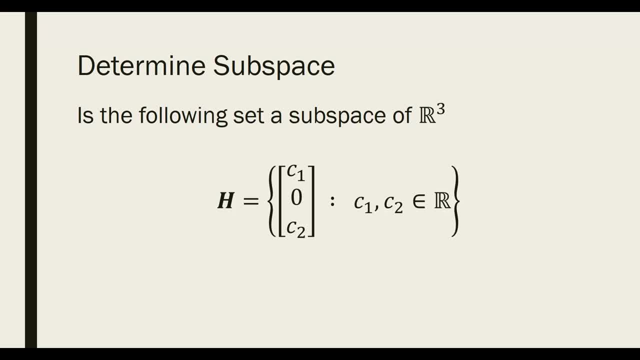 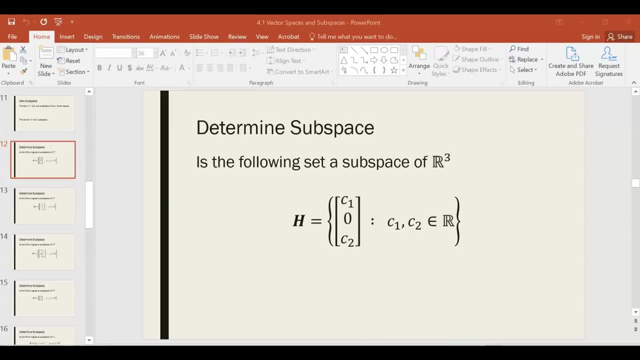 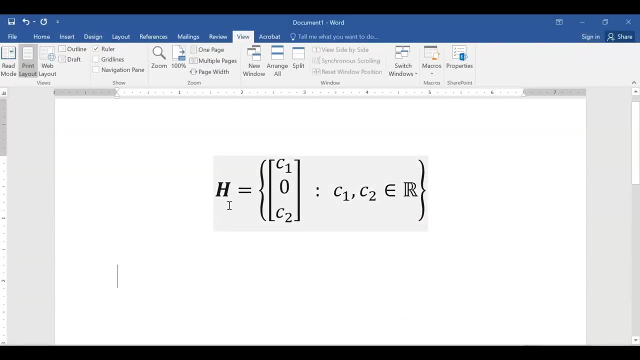 and check that, Alright. so hopefully you've had a chance to do that. I'm clicking out here. So basically we take this h and we're going to see if it's a subspace. So we got three properties. Property one: does it contain? 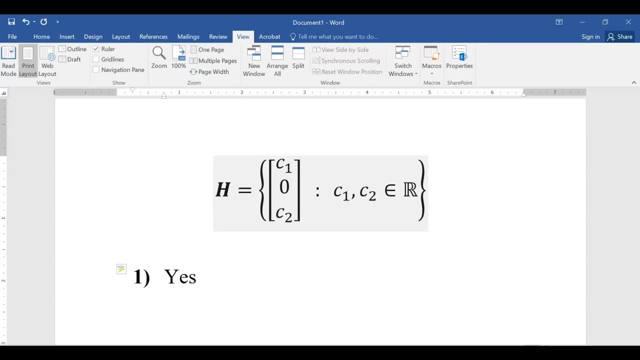 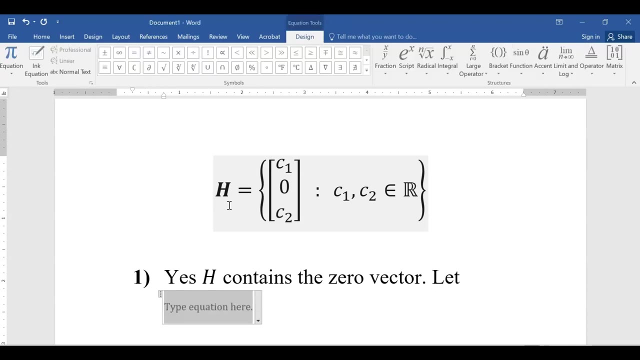 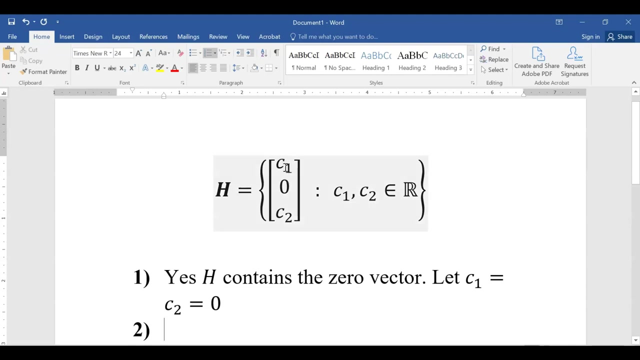 the zero vector, And I say yes, This h contains the zero vector. Basically, all you have to do is let your c1 and your c2 both be zero And you can see that you get the zero vector when you let c1 and c2 both be zero. 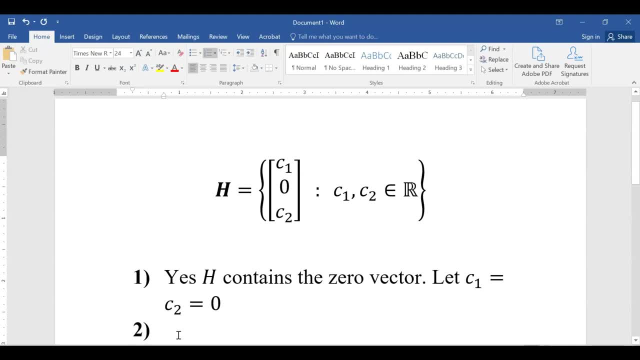 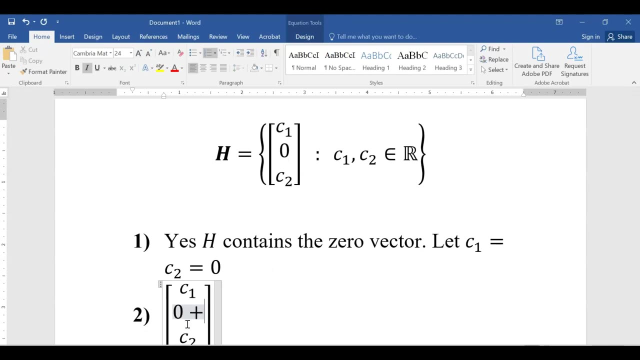 So yes, it contains the zero vector. Second, is it closed under addition, under a vector addition? So what we would do is we'd go up and we'd grab two arbitrary vectors So and test whether the sum whoops. let me scroll down just a bit. 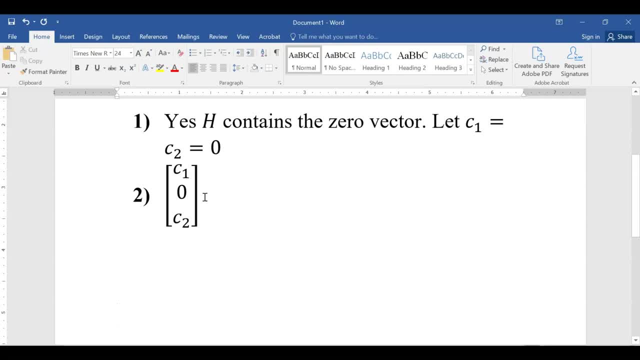 Whether the sum of two arbitrary vectors is in fact also in there. So let's take two arbitrary vectors, I'll call them vector. one which has to look like a1, 0, a2, where a1 and a2 are real numbers. 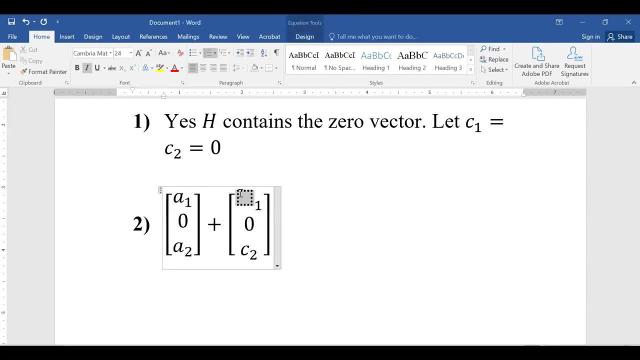 And then vector two. I'm going to use b's here: b1, 0, b2.. Again, one of the b's are arbitrary real numbers. Now, if you add those two up, is it going to have the same form? And the answer is: 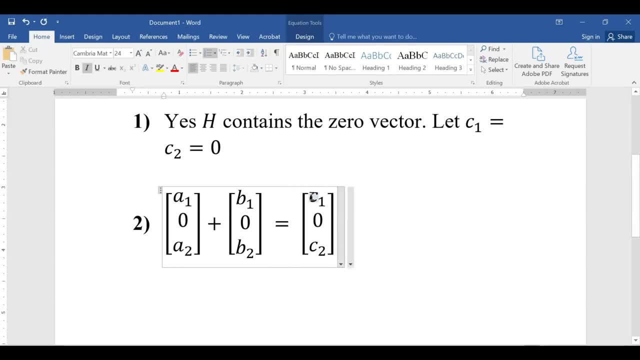 obviously yes, If you add those two things up, you get a1 plus a2, no, I'm sorry, a1 plus b1, and then you get a zero in the middle and then you get an a2 plus b2 at the end there. 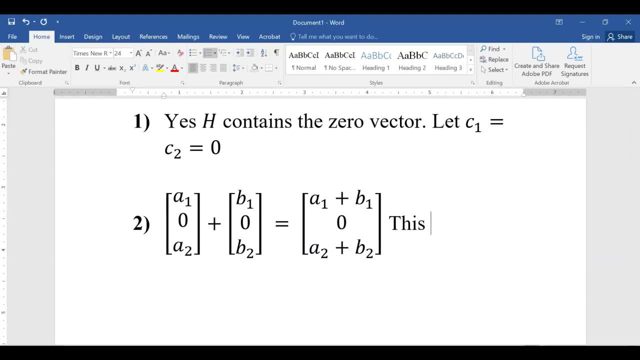 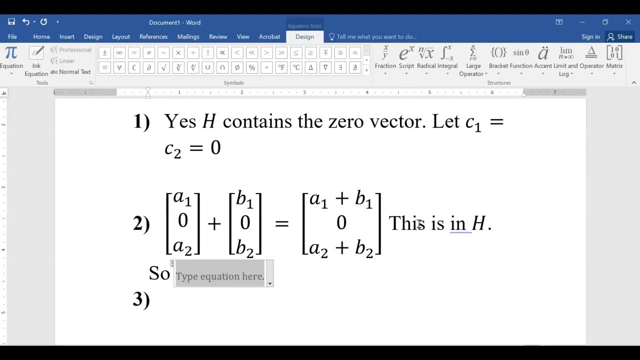 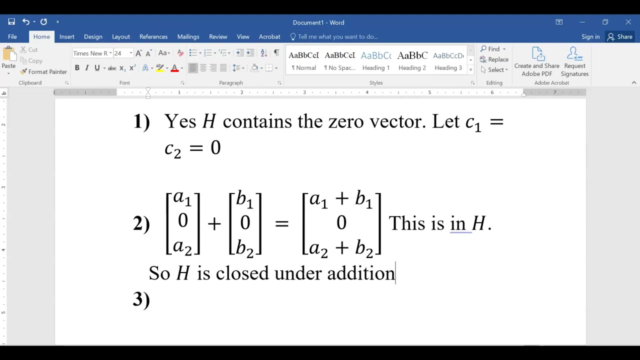 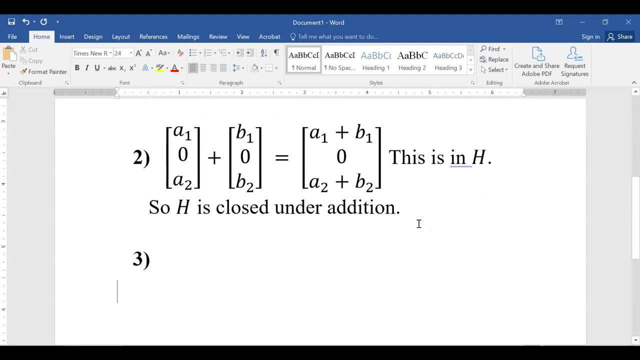 Alright, So this thing is in h and therefore h is closed. under addition, If you add any two vectors in h up, you're going to get a result which is in h. And then, lastly, we want to check to see if h is closed under scalar. 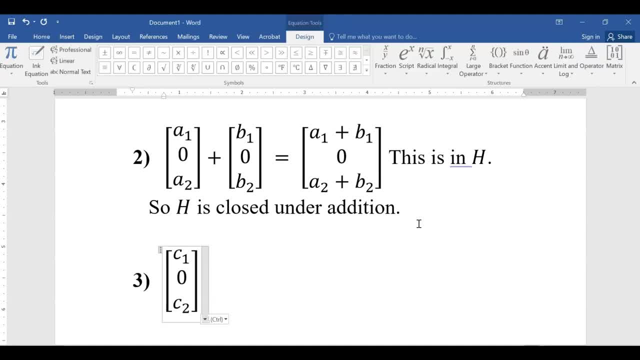 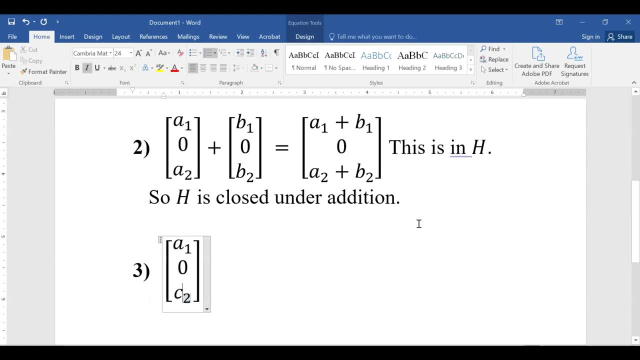 multiplication. So all we have to do is take a scalar multiple times an arbitrary vector. So I'm going to let an arbitrary vector again be a1,, 0,, a2.. If I take a scalar, call it c times that. Well, we know how. 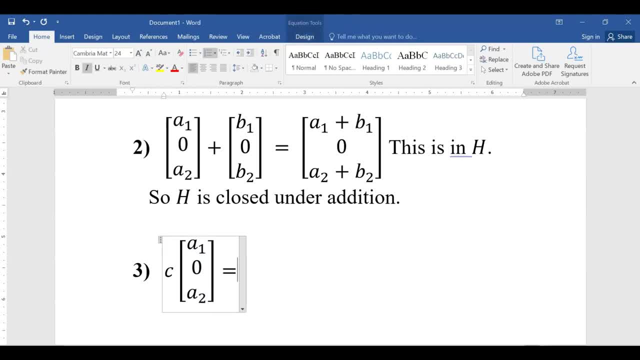 to multiply vectors, times, scalars. We're going to end up with c times a1 in the first spot, 0 in the second spot, And then c times a2 in the third spot, Which does have the form real number: 0 real number. 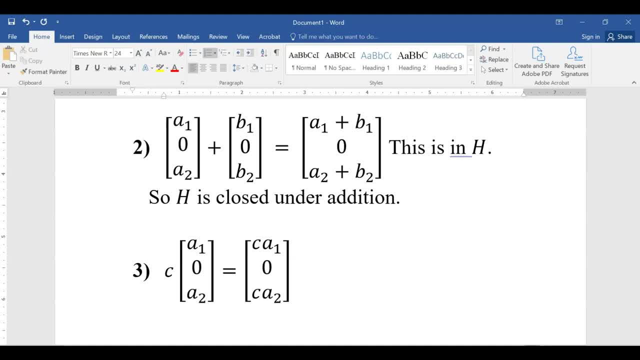 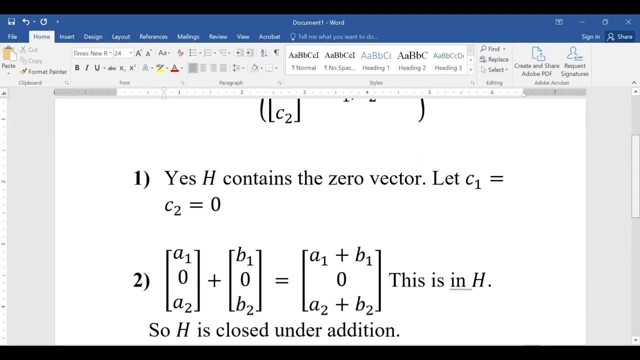 So this is also in h. So whoops. So h is also closed under scalar multiplication. Okay, So h is closed under addition, h is closed under scalar multiplication, And h contains a zero vector. So because all three things are true, 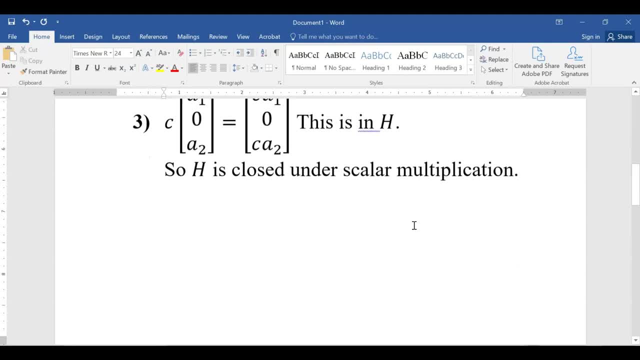 we know now that h is a subspace Of R3.. I won't write of R3. But h is a subspace because it's satisfies all three of those properties. So again remember: closed under addition means that you can add two vectors. 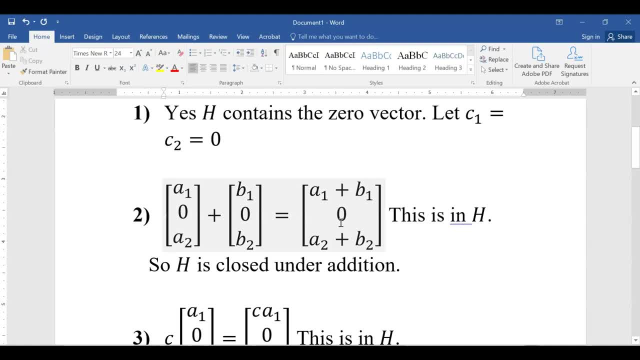 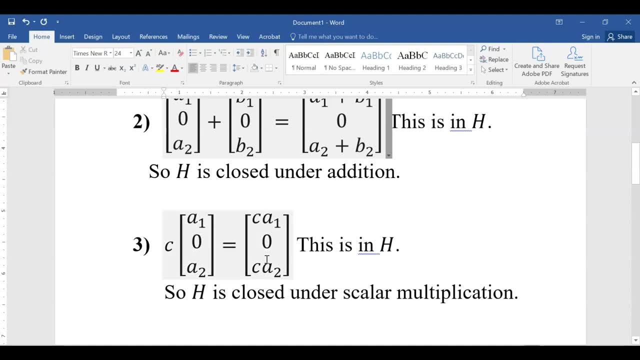 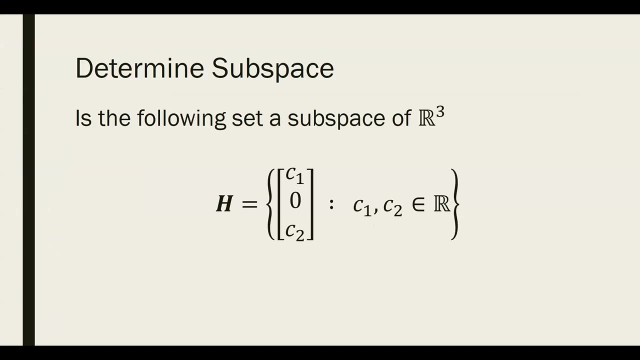 two arbitrary vectors and get back in the same set. Closed under, scalar multiplication means you can take a scalar and multiply times a vector and get back in the same set, Alright. So what I'd like you to do is to take a look at the 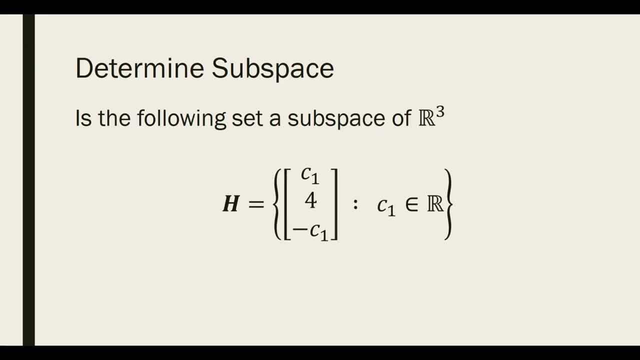 this h and determine if this h is a subspace of R3. Now, this h is not going to be a subspace of R3. And specifically, it's not a subspace because, if you look at the vectors, there's no way to get a zero vector. 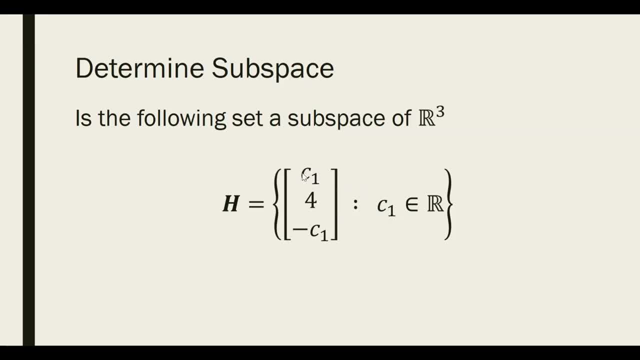 So no matter what I plug in for C1 here I could plug in zero, which would give me a zero in the first entry and a zero in the third entry. But if you plugged in zero for your C1, this middle entry is going to still. 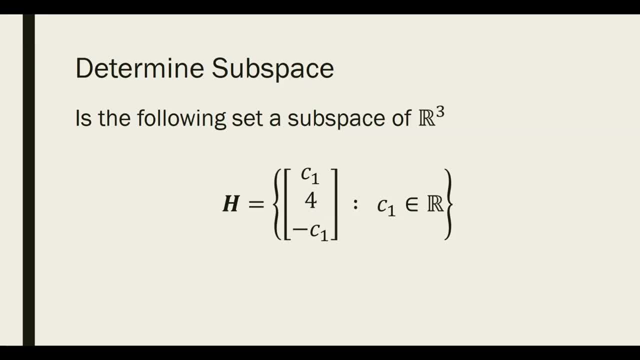 stay four. So this h does not contain the zero vector and therefore cannot be a subspace. How about this one? We have seven times C1, four times C1 and negative two times C1 as the all my vectors are going to have this form. 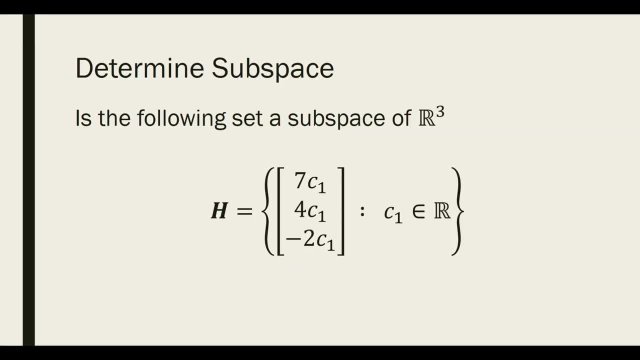 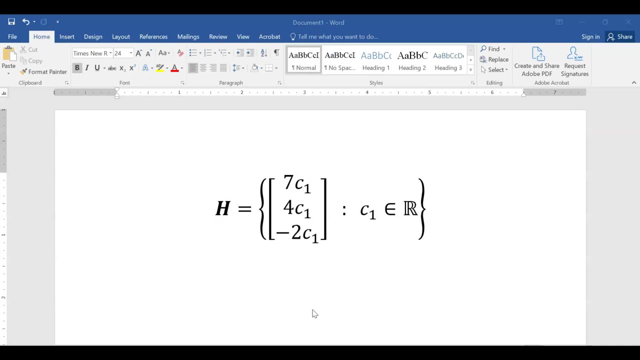 I want you to think if this h can be a subspace of R3.. Push pause on the video. Hopefully you went ahead and did that. I just switched over to the other screen. So basically we go through the process again, So we ask. 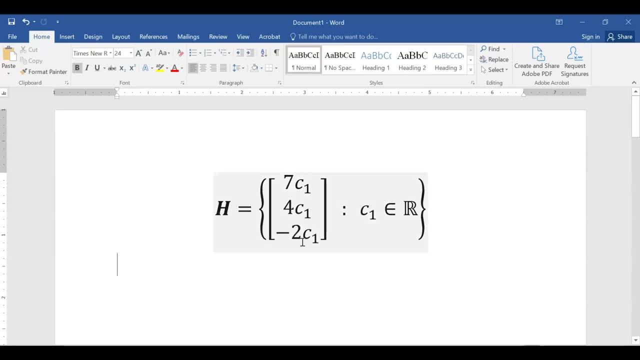 ourselves. first, does h contain the zero vector? And this time it does. If we let C1 be equal to zero, h will contain the zero vector. C1 is zero. We're getting zero as our first entry, zero as our second entry. 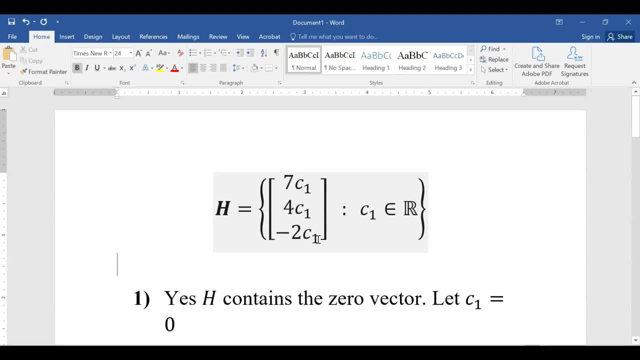 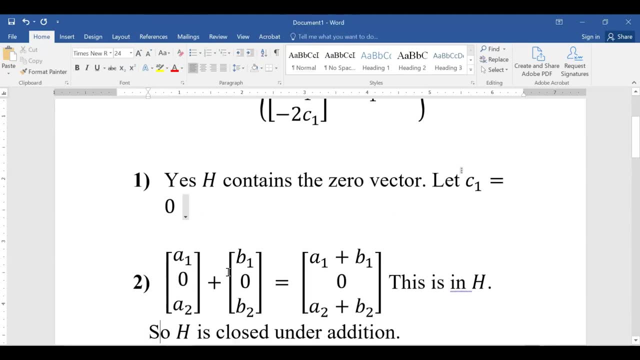 and zero as our third entry. So yes, h contains the zero vector. So we move on. We say, well, what's going to happen when we add two arbitrary vectors? Now, this is what we did last time, but it's the same. 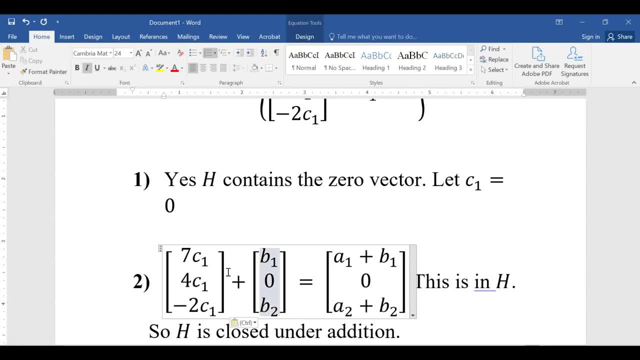 type of principle. We're going to take an arbitrary vector. I'll probably relabel some of these things and add another arbitrary vector. So let's take A1, A1, A1 and then B1,, B1,, B1, so that we're not 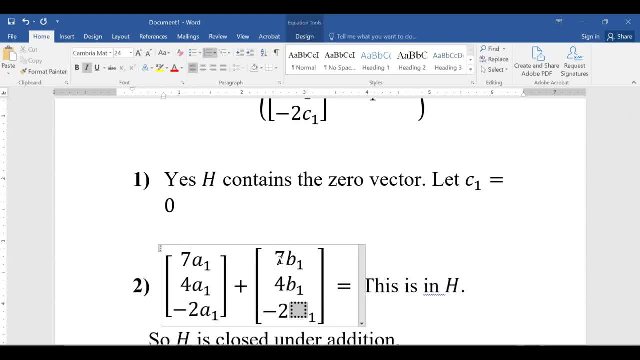 using the same letter. So if you add two arbitrary vectors, what you end up with is 7A1 plus 7 times B1, and then you get 4 times A1 plus 4 times B1, and then you get negative 2 times. 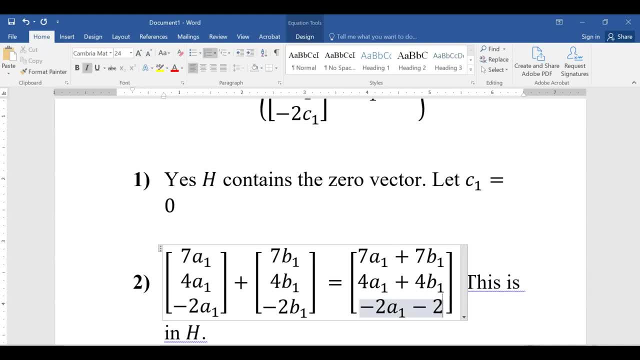 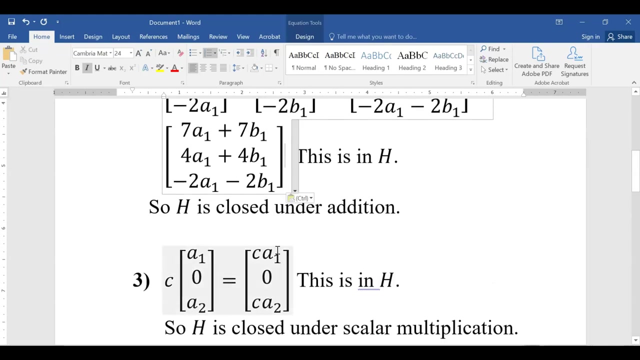 A1 plus negative 2 times B1. alright, Rewriting this. let me rewrite this. what you're going to see is that this does have the form that other vectors in H are going to have. It's going to look like 7. 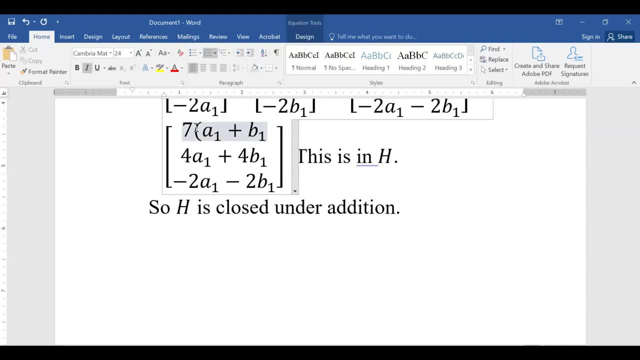 times A1 plus B1 and A1 plus B1, since it's a sum of real numbers, is just a real number itself: 4 times A1 plus B1. again, all I'm doing is factoring out the 7, factoring out the 4. 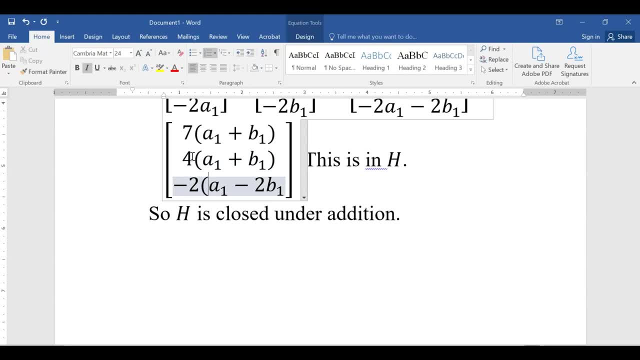 and then negative 2 times A1, and this will be a plus B1 when I factor out a negative 2.. So you can see this vector also has the same form. It's 7 times a real number, 4 times that same real number. 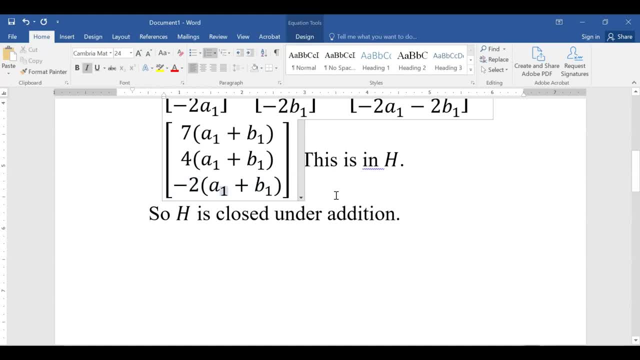 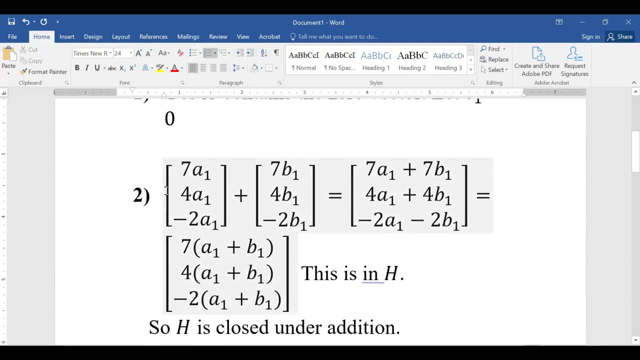 and negative 2 times that same real number. So this has to be in H and therefore H is closed under addition. Now, lastly, what we're going to do is we're going to say: well is an arbitrary vector times, an arbitrary scalar, also in H. 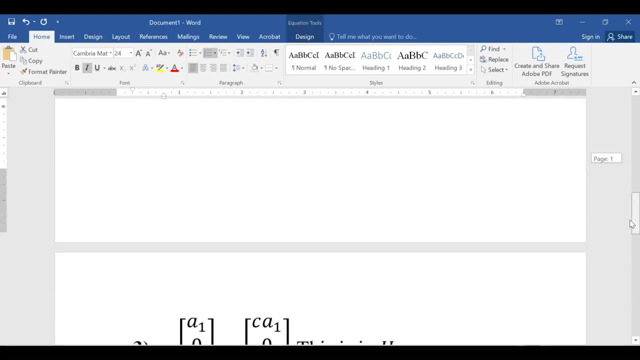 In other words, is H closed under scalar multiplication. So we're going to take an arbitrary constant, multiply it times vector 7, A1, 4 A1, negative 2, A1, and we're going to get 7 times C, A1 and then 7. 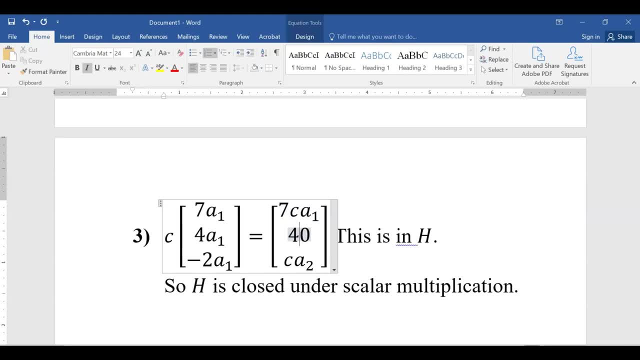 no, I'm sorry. then 4 times C A1, and then negative 2 times C A1 and notice, just looking at this, this is going to be 7 times a real number, 4 times a real number, in fact, that same exact real number. and then 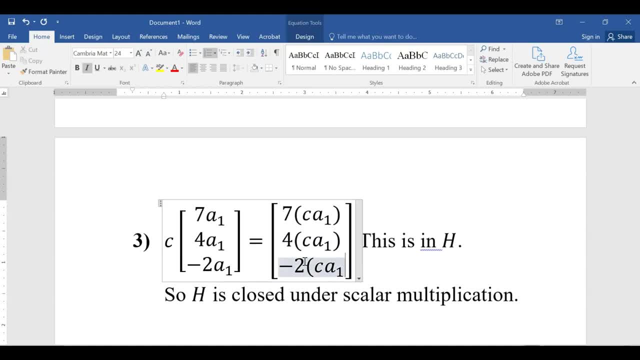 negative 2 times that same exact real number. So it looks like 7 times a real number, 4 times a real number. negative, 2 times a real number. Therefore, this thing has the form that it has to have to be in H. 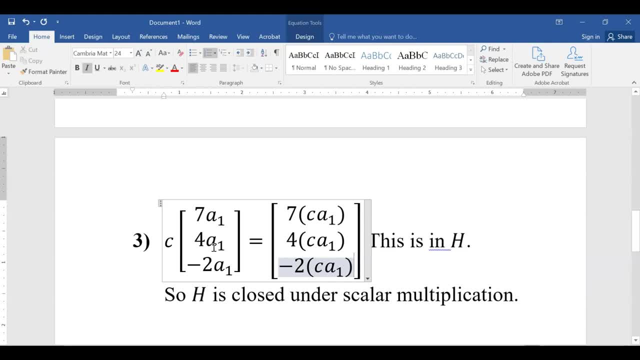 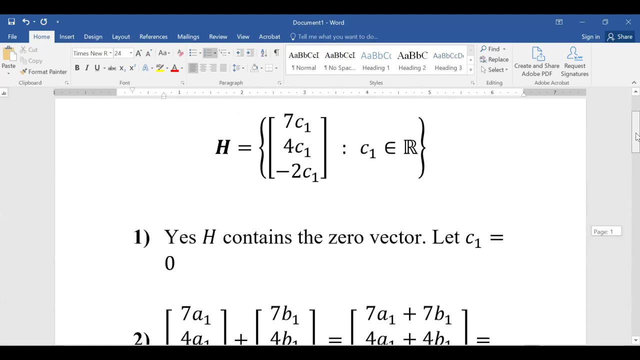 So this vector, when you multiply scalar times an arbitrary vector in H, you land back in H. So that means that H is closed under scalar multiplication. So we see that H contains the zero vector. H is closed under addition and H is closed under scalar multiplication. 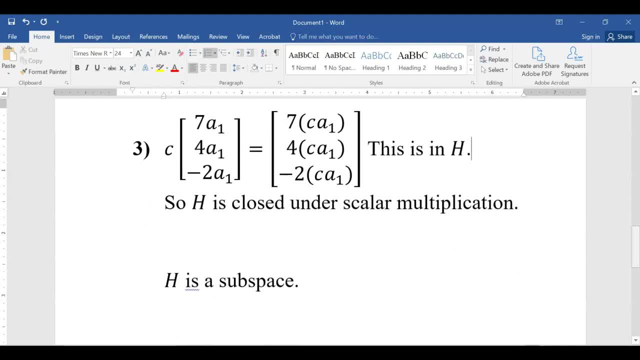 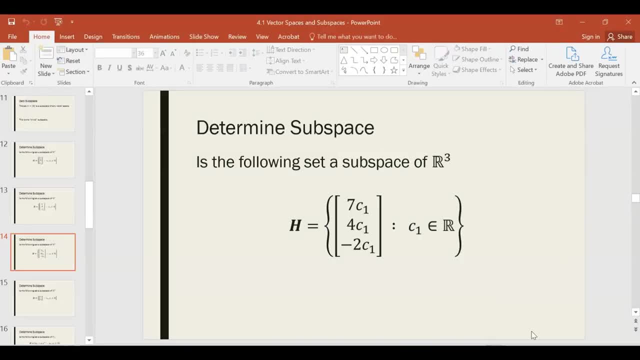 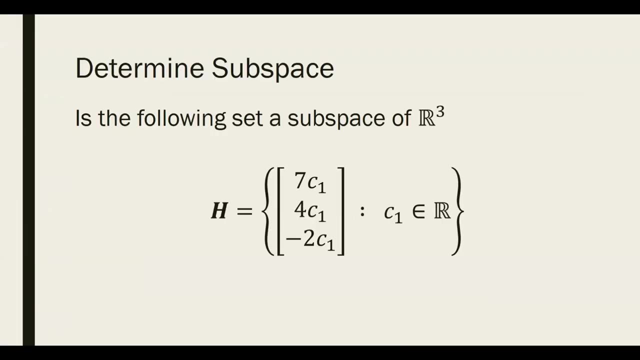 therefore, H has to be a subspace, And that's it. So H is, in fact, a subspace of R3.. Now, one little tricky thing that you do have to watch out for a little bit is a question like this. It says is the following a. 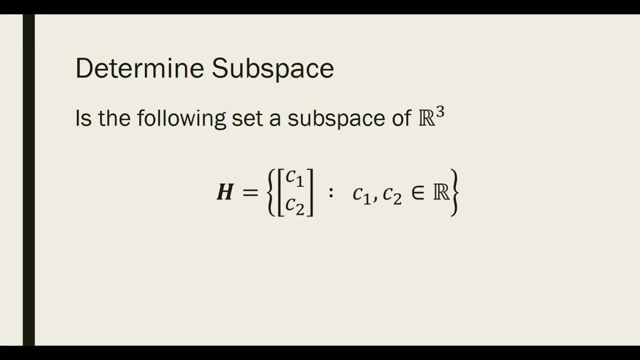 subspace of R3?? The answer to this is no. The answer to this is no, Not that it's not a subspace. it's a subspace, but this one is a subspace of R2.. So just be careful about that R3. 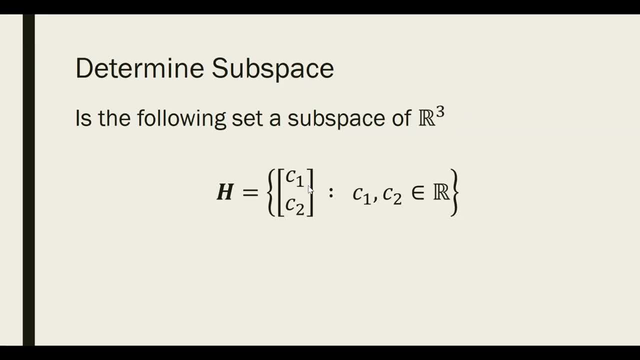 has to have vectors with three entries. This one only has vectors with two entries. So this is not a subspace of R3.. However, it would be a subspace of R2.. Hopefully that makes sense. So when we say subspace, it does have to contain the right. 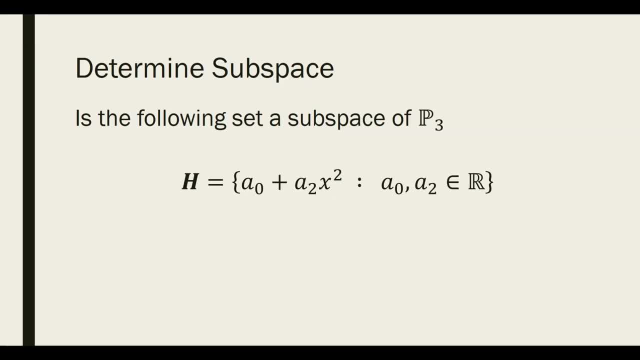 size vectors. Now we can expand our knowledge. let's say and figuring out: well, is the set of these vectors a subspace of polynomials of degree 3 and less? Okay, So we have a set here which contains basically a1 plus a2 times x2. 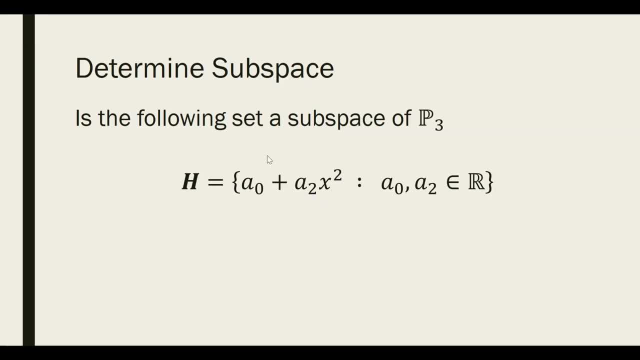 so all of the polynomials in this set are going to look like a constant plus something with a squared component. Now the test for subspace doesn't change. We still have to figure out. does this contain the zero vector? Does this contain? excuse me, 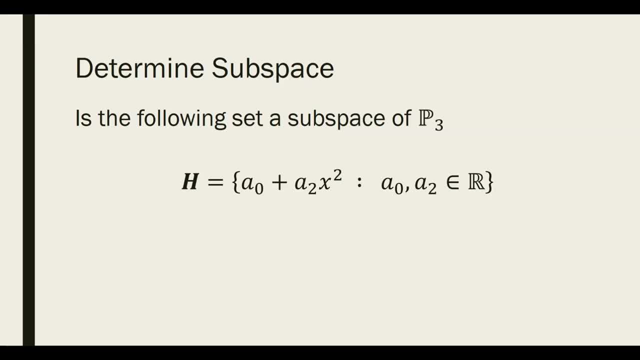 does this contain the zero vector? first, Is it closed under addition? Is it closed under scalar multiplication? So we check those three properties again. I want you to push pause on the video and see if you can check those three properties and then I'll come back. 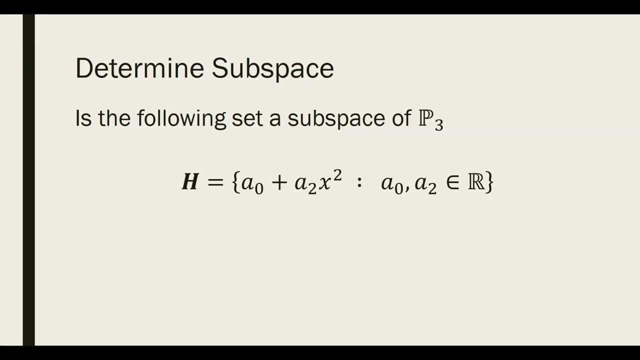 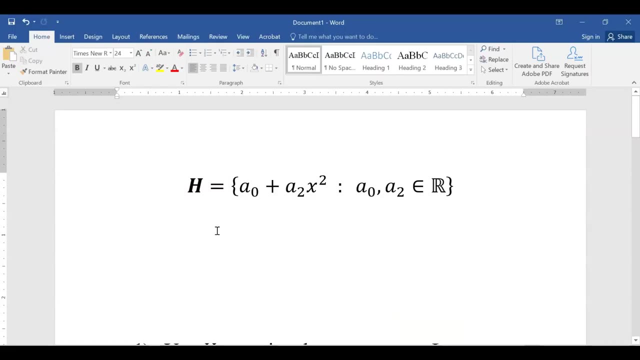 and go through them. Alright. so hopefully you went ahead and did that and checked that out. So let's go pull up our subspace there and say, or our set or hope it's a subspace. So we check the three properties First: does h contain the zero vector? 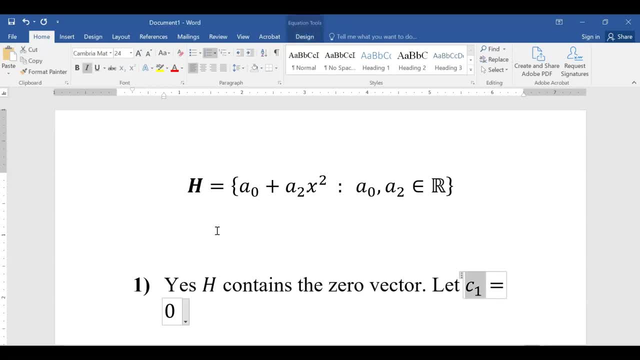 Yes, it does. All we have to do is let our two coefficients, let the a sub zero. by the way, the reason I'm denoting this as a sub zero, it's the real number coefficient on the x to the zeroth power. a two is the real number coefficient. 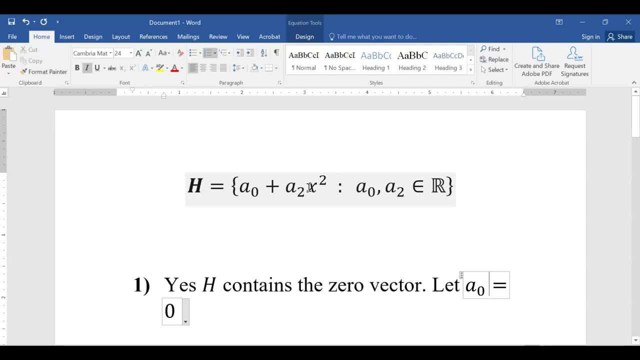 on x to the second power. so I'm trying to match them up that way. So if we let a sub zero be zero and let a sub two be zero, then you'll notice that h does contain a zero vector. and again, the zero polynomial is just a polynomial with all zero coefficients. 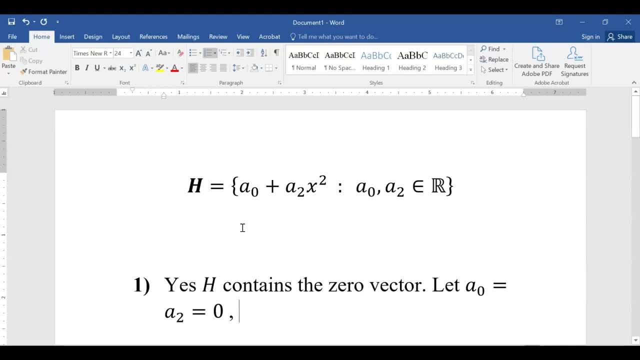 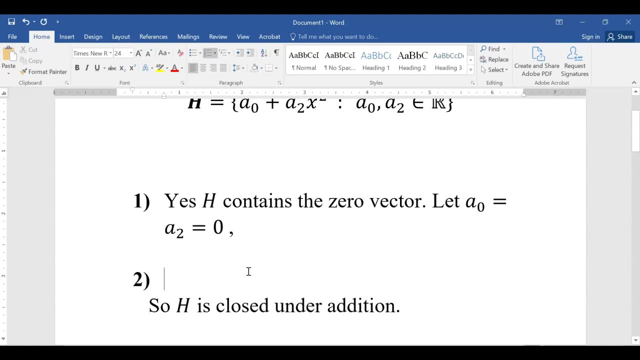 I didn't mention that before. So there you go. h contains a zero vector because it contains the zero polynomial. Let's see if h is closed under addition. Let's say: I have a polynomial that has real number coefficients, that looks like that, and another. 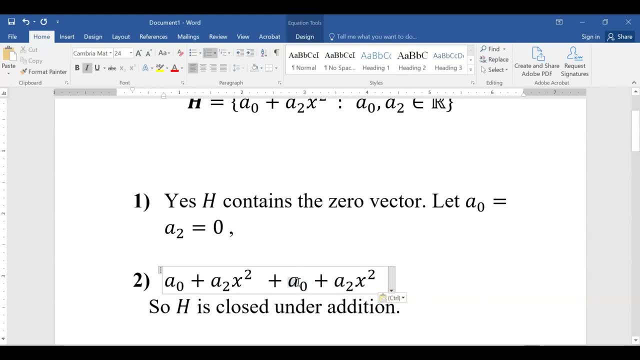 polynomial who has real number coefficients that look like that. Let me switch up my coefficients letters there. So we have this first polynomial if you add it under normal polynomial addition to a second polynomial of that form. the question is: are we going to get a third polynomial which has that form? 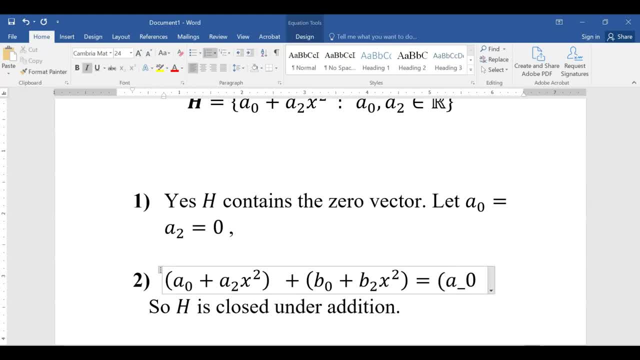 And the answer is yes, we are, because when you combine like terms a zero plus b zero combines and gives you a real number coefficient. and then when you combine like terms a sub 2 x squared and b sub 2 x squared, you're going to get 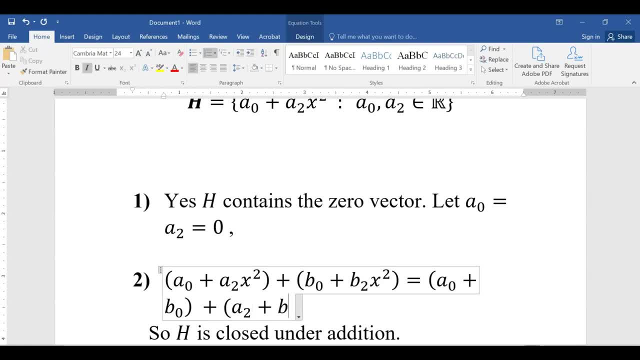 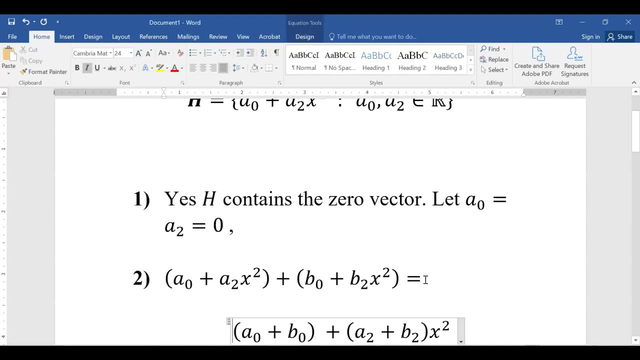 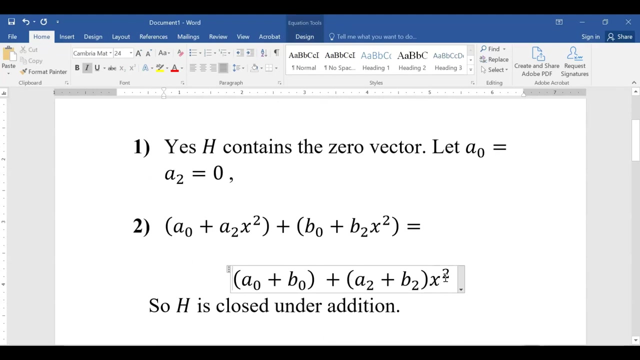 a sub 2 plus b sub 2 times x squared. Let me just take our and, and there we go. So when you add them you still get that same form. you get real number constant plus some coefficient times x squared. So yes, h is closed under addition. 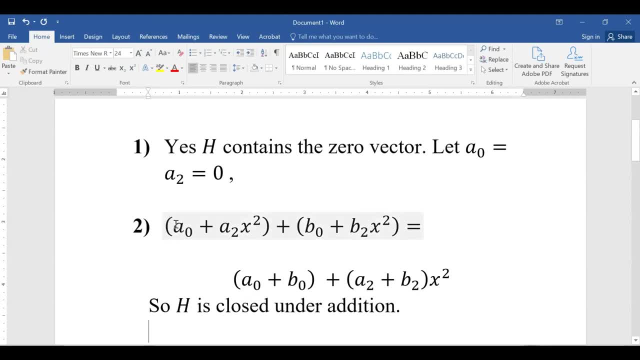 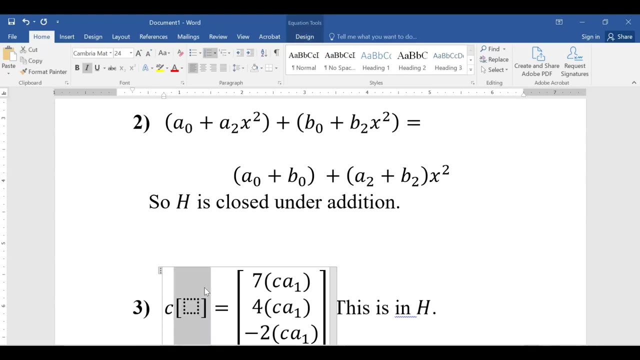 And in a similar way, if you take a look and you do the same thing, you should multiply scalar times an arbitrary vector. Let's in fact do that. so scalar times an arbitrary vector. ah, by the way, be careful about this. we have to take the scalar, has to. 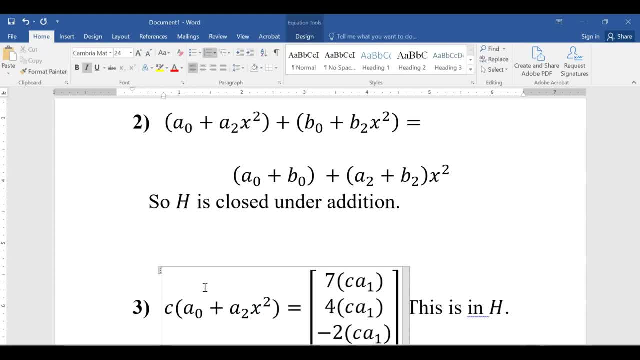 distribute, multiply the vector, the entire polynomial. well, you're going to get c times a, zero plus c times a, two x squared, and yes, this in fact is an h. and because it's real number, constant, plus some real coefficient, times x squared, so that's an h. so h is closed under. 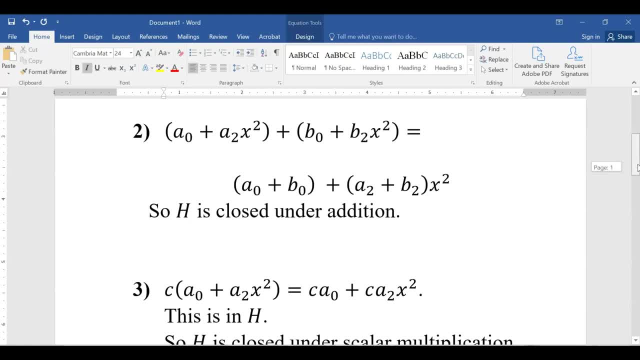 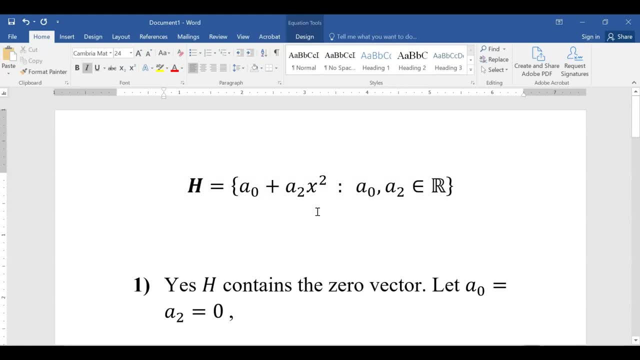 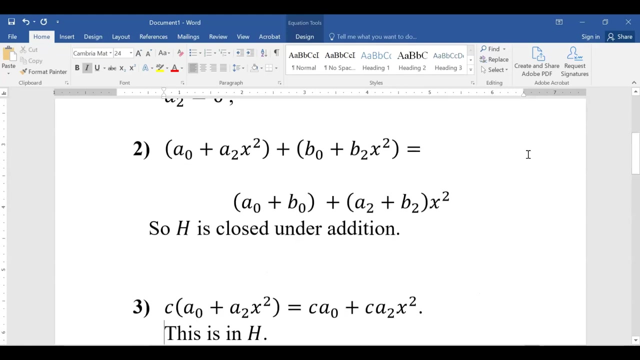 scalar multiplication. so we've just shown that all vectors of this form form a subspace of polynomials of degree three and less. because it this, all polynomials of this form contain the zero vector. all polynomials of this form, when I add them, will still be of that. 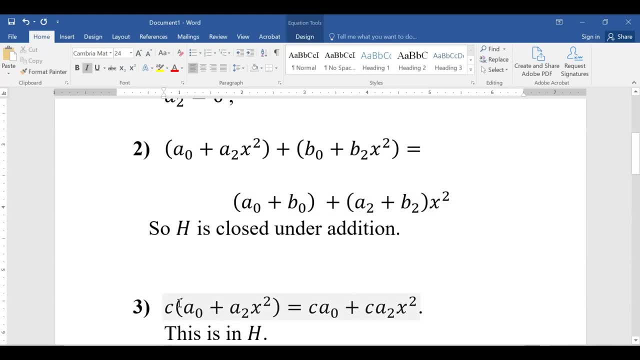 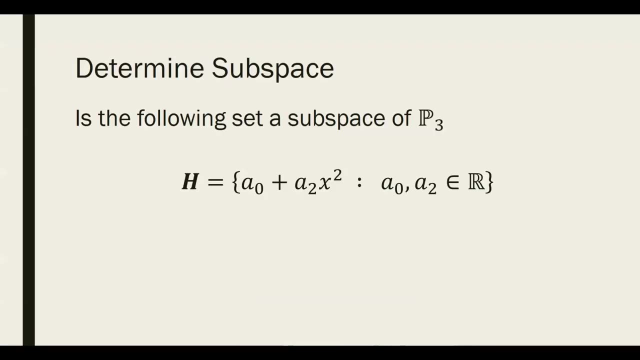 form and all polynomials of this form. when I take a scalar and I multiply it, it's still going to be of that form. so because all three of those things hold true, h has to be a subspace of polynomials of degree three and less. I want. 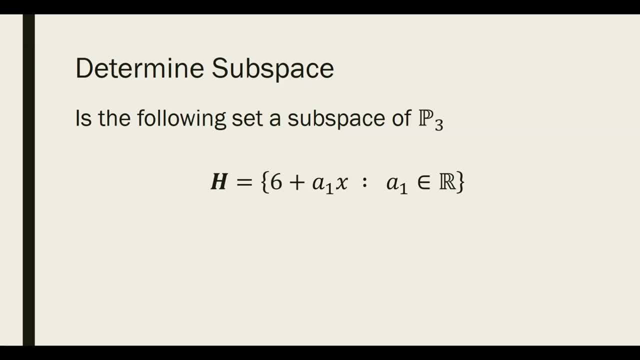 you to think through this, set this h and decide if this h is going to be a subspace of polynomials of degree three and less. push pause on the video if you need now. the short answer here is that this is not a subspace, okay, you. 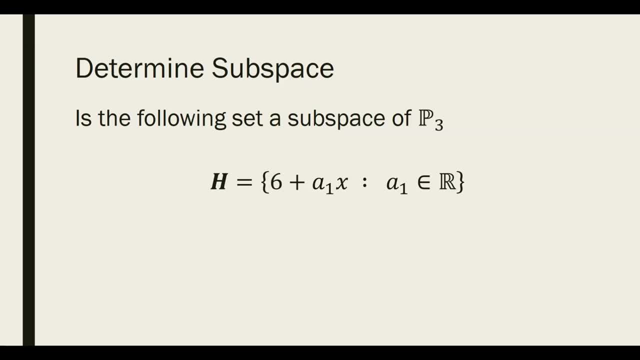 can prove that in a number of different ways, but probably the easiest way to prove that is that this does not contain the zero vector. the best I can do is letting a1 here be zero. if you let a1 be zero, the coefficient times x becomes zero times x. that goes. 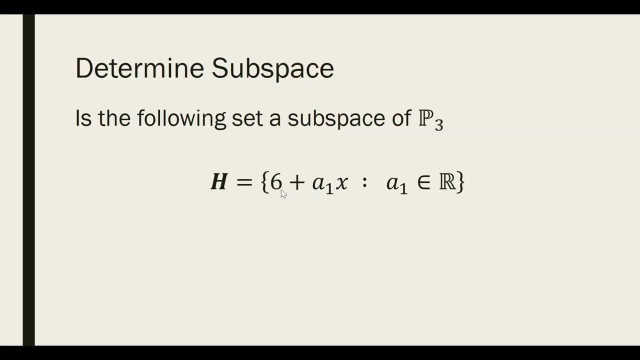 away, but I still have a six remaining, so I can't have these plus sixes or plus twos or anything like that around if I wanted to have an actual subspace. so this is not a subspace of p3 because it does not contain the zero vector. 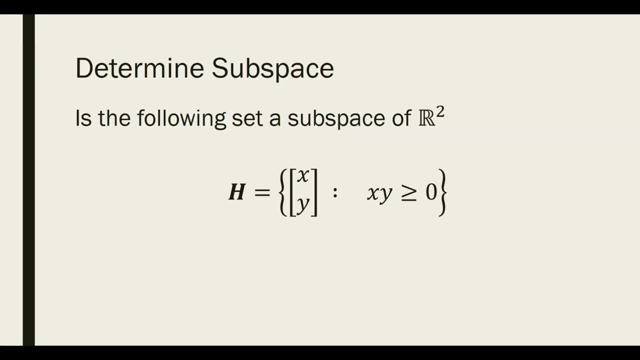 okay, I want you to think about this. here's a unique set. take all of the two dimensional vectors whose entries, when we multiply them, give me a positive number. so if I take a positive and positive, that would be in this set. if I take a negative number, 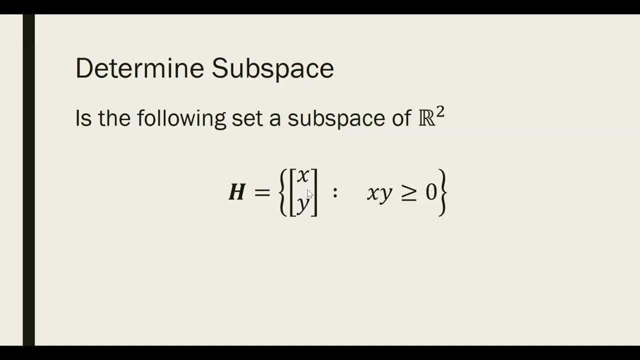 times a negative number. that would be in a set. I shouldn't say that if my negative number is in the first entry, negative number is in the second entry. that would be in the set. I want you to push pause and think through if this actually is a subspace. 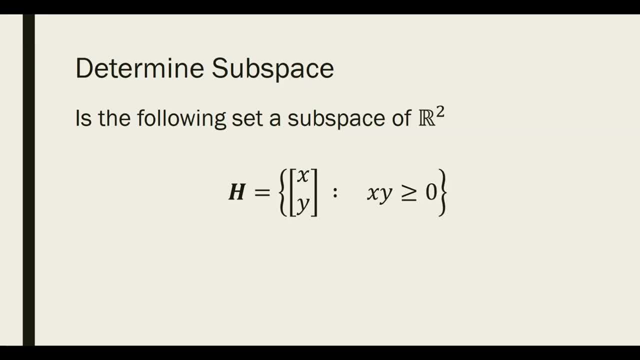 of r2, alright, so this one's a little bit trickier, um, because it's not a set that we deal with a whole lot, um, basically, if you want to think of it, think of these vectors as points in r2. this would be like the first and 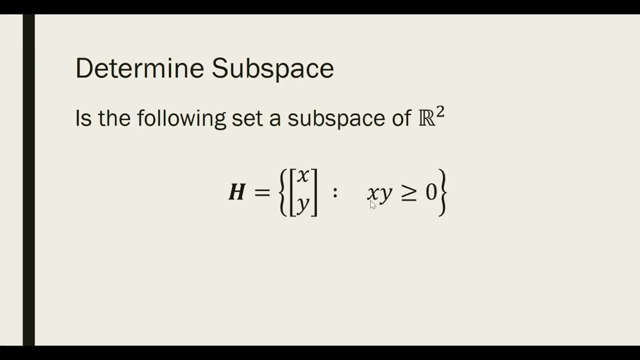 third quadrant combined. okay, we either have positive: positive, that gives us a, you know, greater than or equal to zero, or we have negative: negative, which gives us greater than or equal to zero, or one of them has to be zero, either the x or the y, or both. 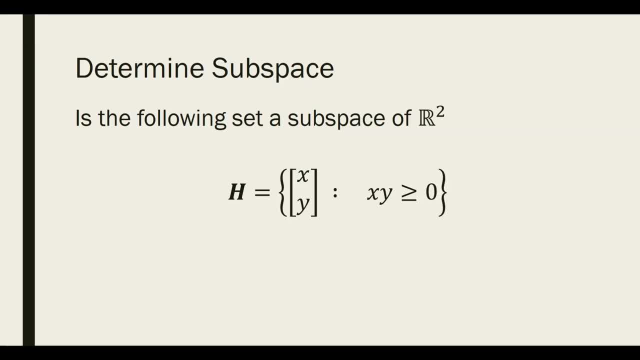 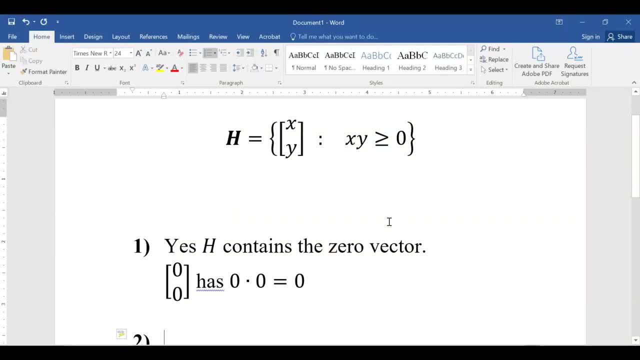 so what you'll find is that, first off, if you're going to um utilize the properties of subspaces that we looked at, we ask first: does this contain the zero vector? and yes, it does, because- notice that the zero vector- we have zero, zero entry if we multiply the first entry. 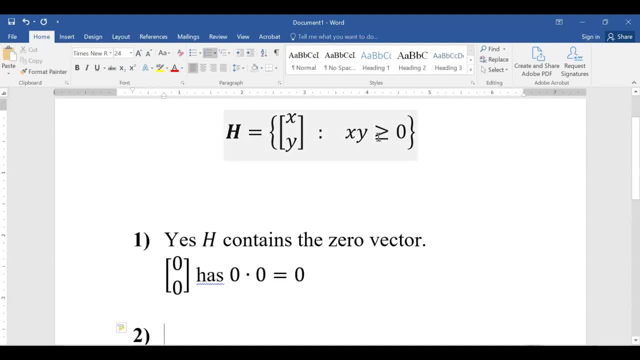 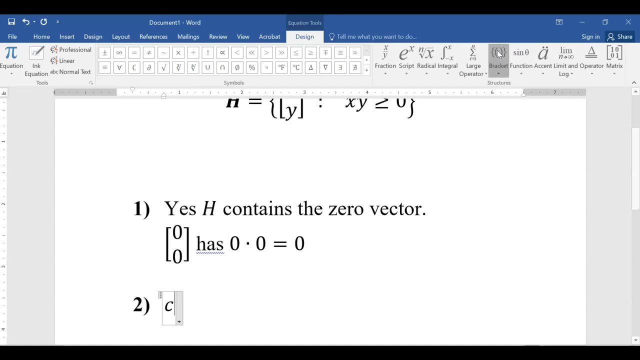 times the second entry, we get back a zero. since zero is greater than or equal to zero, then yes, h contains a zero vector. now also, what we'll notice is that if you take a scalar and you multiply it, whoops times any vector in here. my apologies. 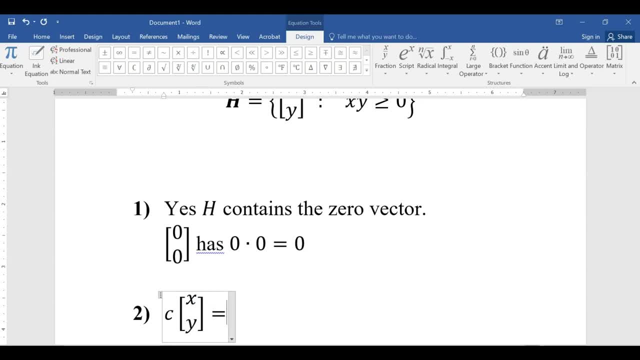 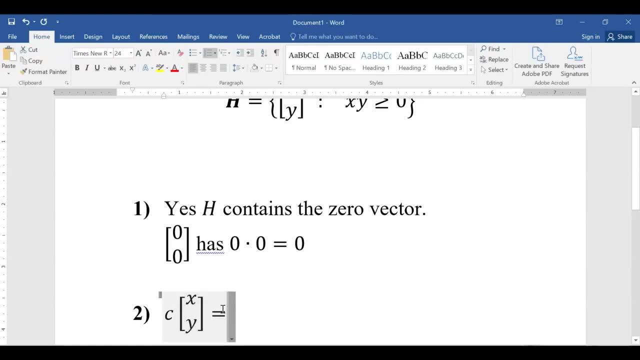 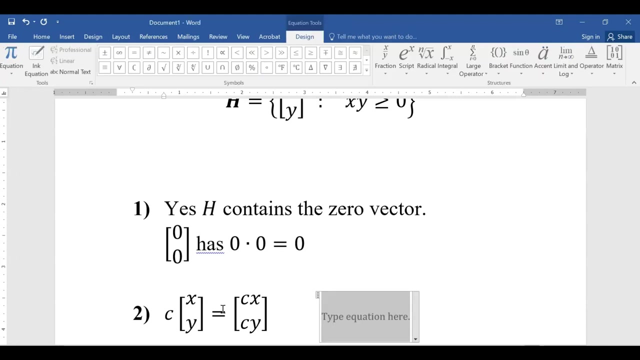 so if xy is a vector in h, what you'll see is that multiplying by a scalar will give you cx in the first entry, cy in the second entry. now think about what would happen if you took the first entry of this new vector and you multiplied it. 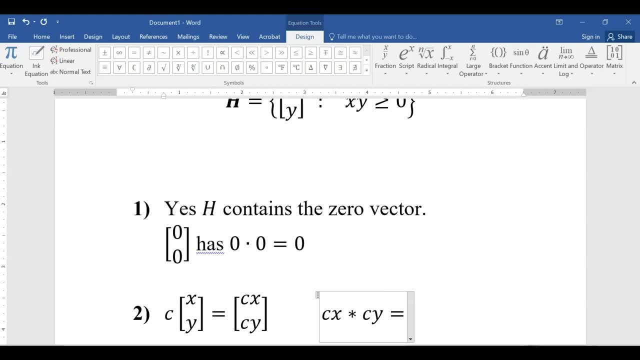 times the second entry of this new vector. what you're going to end up with is a c squared times x times y. now, c squared is obviously positive or zero, depending on whether c is non-zero or just zero. so it's going to be positive or zero. 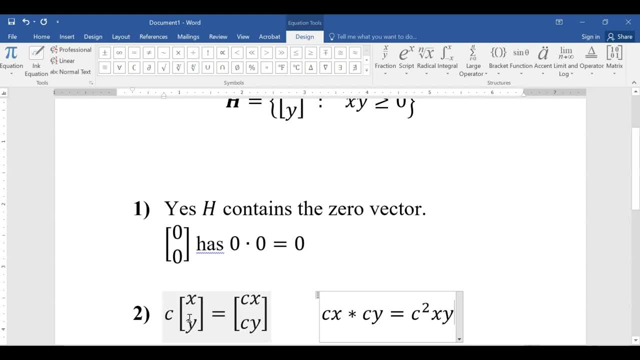 and we already knew we started with this xy in h, so we knew that x times y is positive. so what we're ending up with is a positive times a positive- or at least a positive times a zero- vector which is in fact greater than or equal to zero. 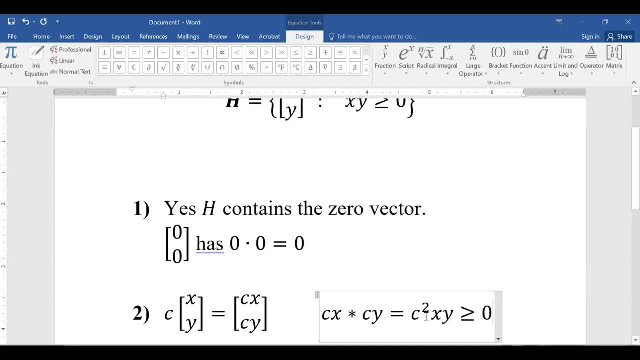 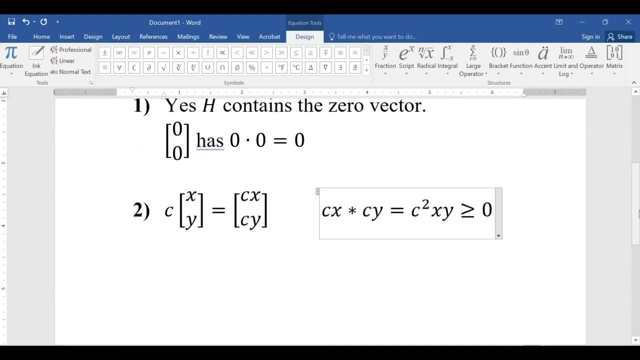 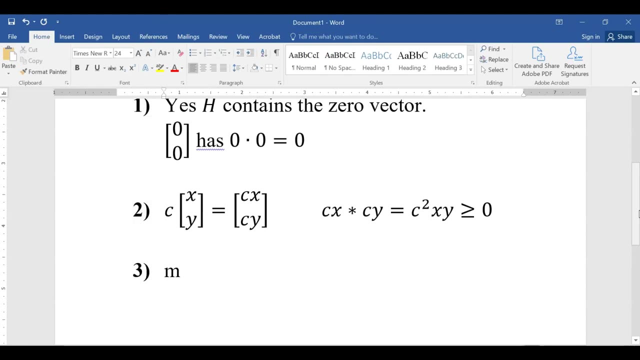 so think about it as positive times positive, or maybe a better way to say that is: non-negative times non-negative. so non-negative times, non-negative. so this group is in fact closed under this set is closed under scalar multiplication: alright. now the trouble is the additive property. 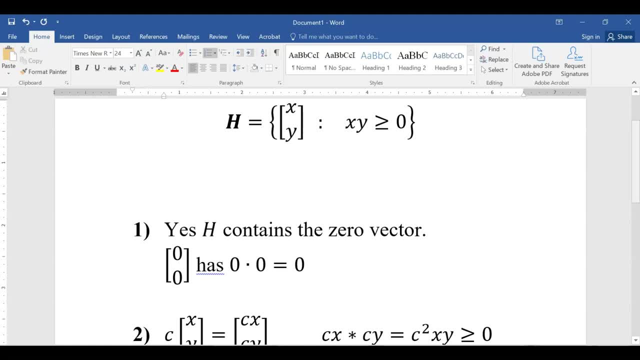 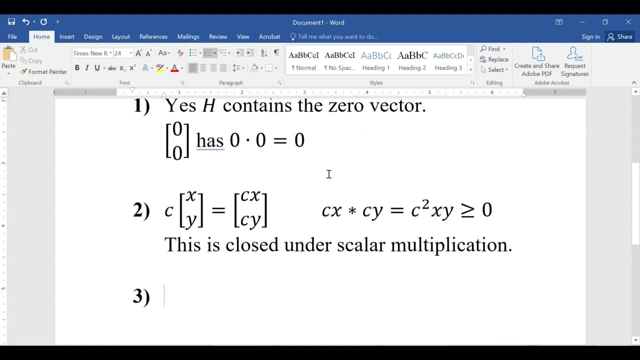 it turns out, if you add two vectors whose entry is multiply to give you something non-negative, then their entries don't necessarily have to multiply to give you something non-negative. let me give you an example. so if I took the vector, let's say two zero, and then 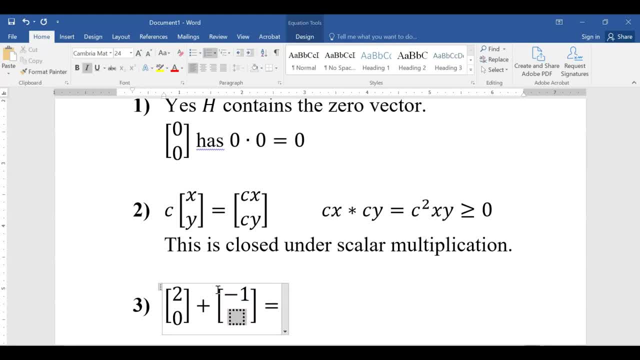 I added the vector negative one, negative three. what you'll notice is that two times zero gives us a non-negative number: negative. one times three gives me three, that's a non-negative. so each one of these individually is in fact in my set H, but when you 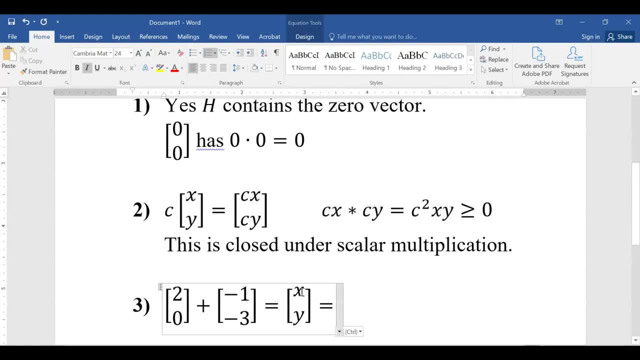 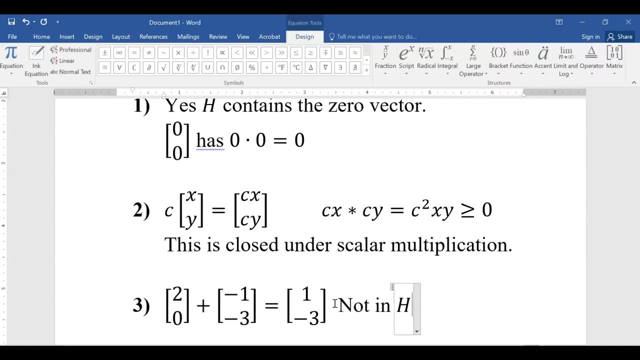 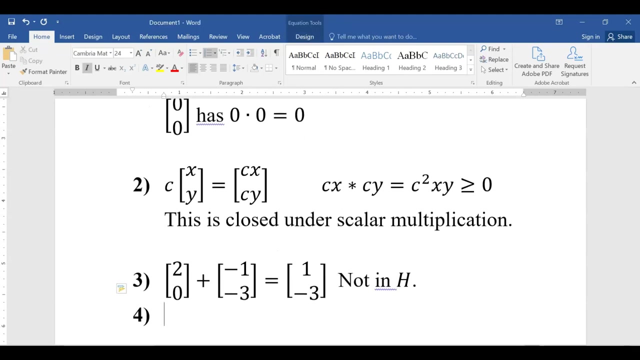 add them, you get a. one is the first entry and a negative three is the third entry. one times negative three is not in H. so even though this H contained the zero vector and even though this H was okay with scalar multiplication, this was not okay with vector addition. 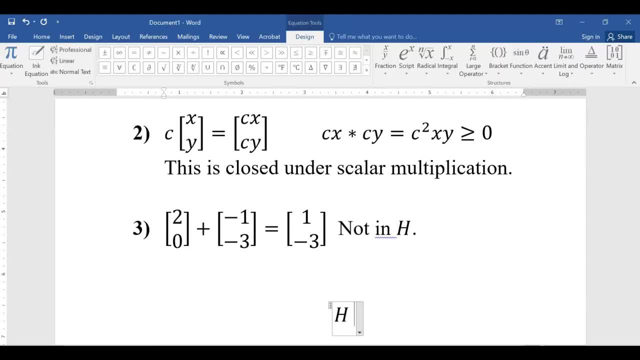 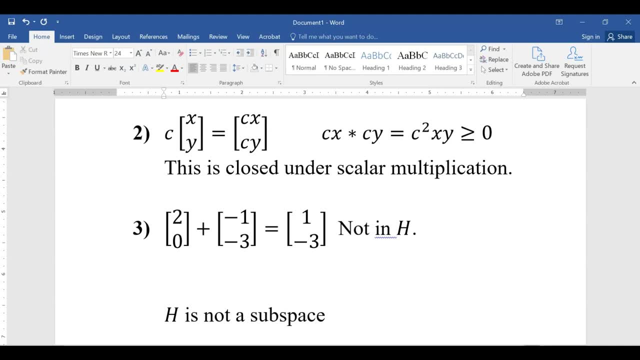 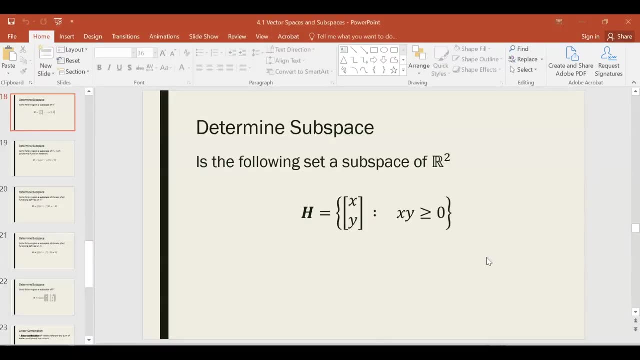 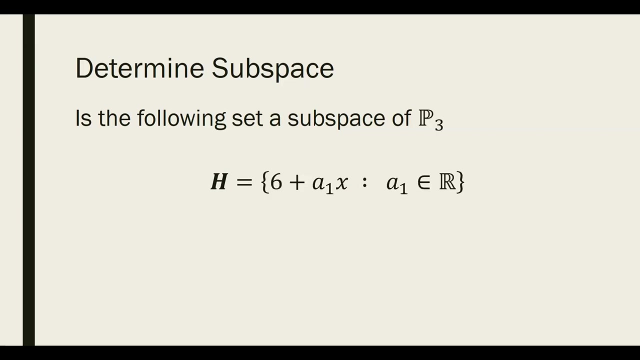 so H, in this case, is not a subspace of R2. alright, so there you go. so this H is not a subspace of R2. now, what we're going to do here. we've seen a bunch of subspaces, different types, from R3, from polynomials. 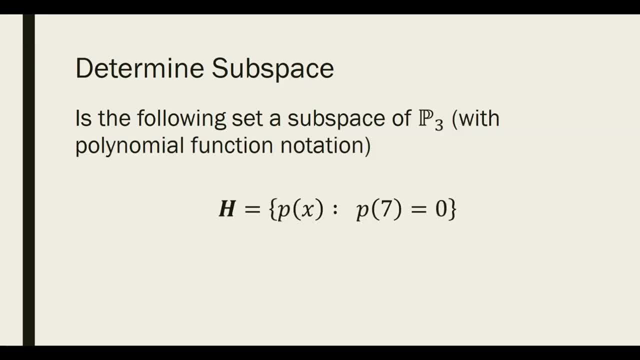 from an R2 example. I want you to look at another, slightly different example. so what we're going to do is we're going to change the notation slightly on our polynomials and we're going to say, instead of thinking of these polynomials as being sums, 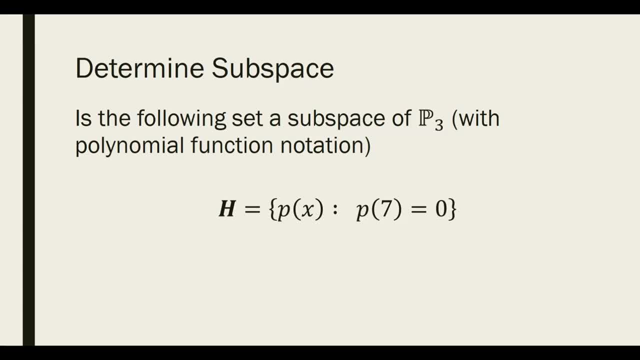 of a coefficient, plus X to the first, plus X to the second, plus X to the third. I'm going to think of these polynomials as being polynomial functions, alright, and we can interchange the polynomial versus polynomial function pretty quickly, so hopefully that makes sense what I'm saying there. 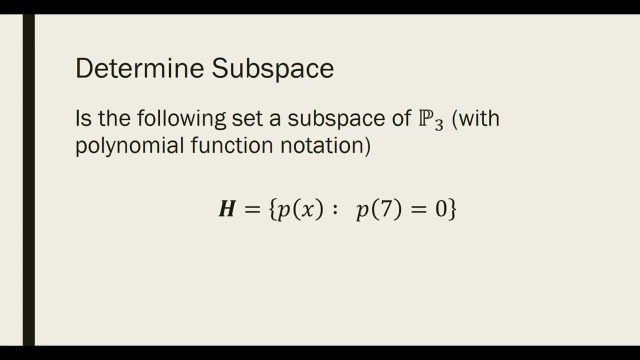 so is this following: set a subspace of polynomials of degree three or less. and again, I'm using polynomial function notation, so I think probably what would be best is if I actually explain this a little bit more in terms of this notation. this is basically saying: 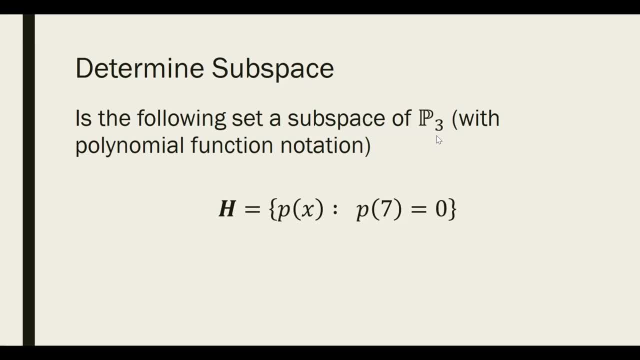 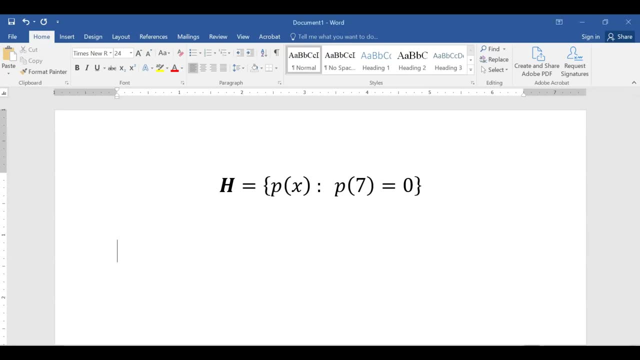 all polynomials of degree three or less, that when you plug in seven you end up getting out zero. alright, so here's my age. so what I'm trying to get at is these polynomials in here are, for example, something like: the polynomial P of X equals. 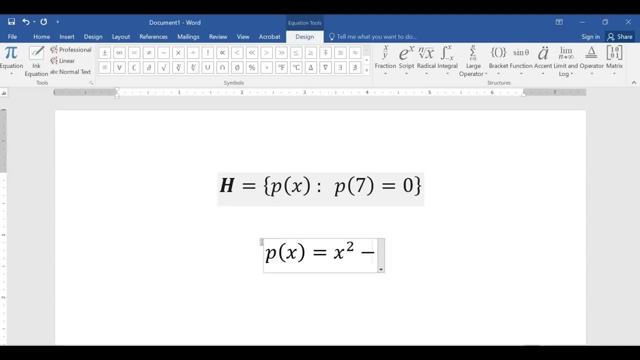 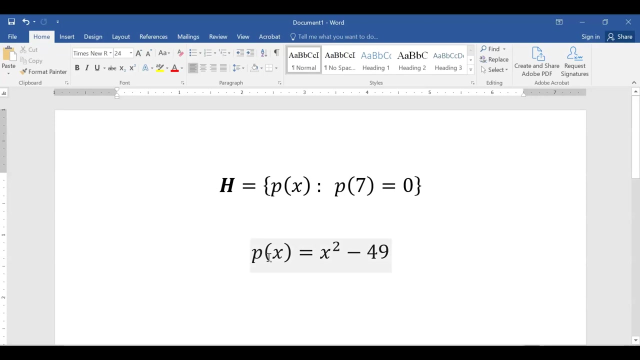 X squared minus forty nine. X squared minus forty nine is a polynomial of degree three or less. that when you plug in seven you end up with a zero. alright. so P of X would. this polynomial would be in H. now there's a lot of other polynomials that would be in H as well. 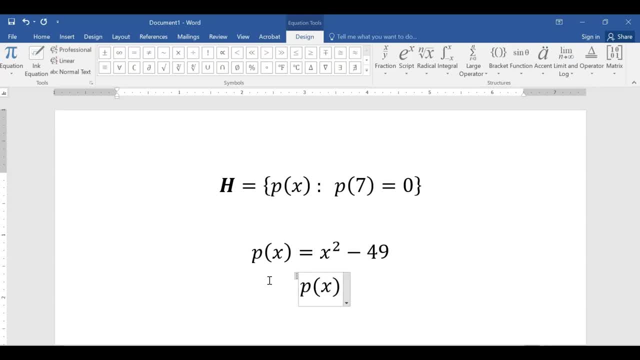 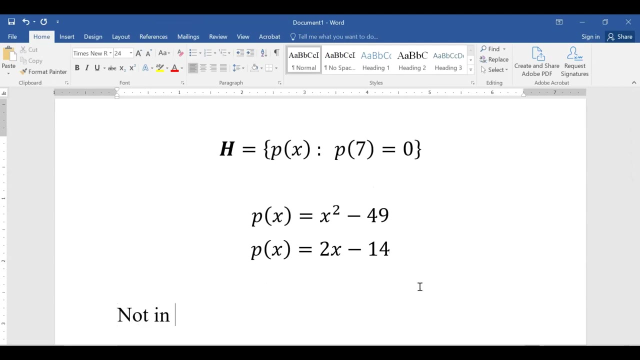 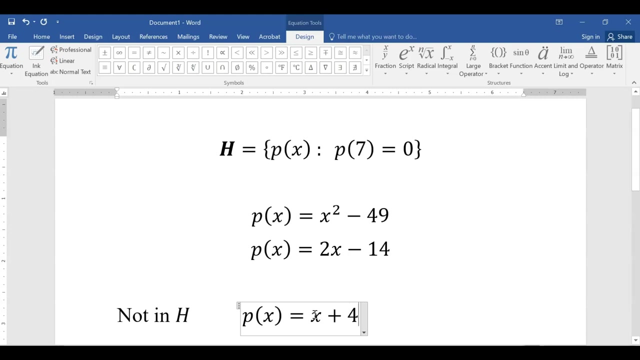 take a polynomial like we'll just take two X minus fourteen, that would also be an example of a polynomial in H um. a polynomial not in H? um would be any polynomial such as P of X equals X plus four. if I plugged in seven into this polynomial, 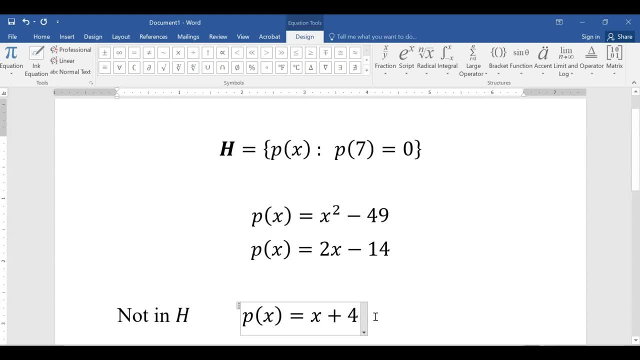 seven plus four is eleven. obviously it's not zero and therefore this polynomial would not be in H. so that's what we mean with this notation. it's all the polynomial functions, so that when you plug in seven you get zero, and if you plug in seven and get 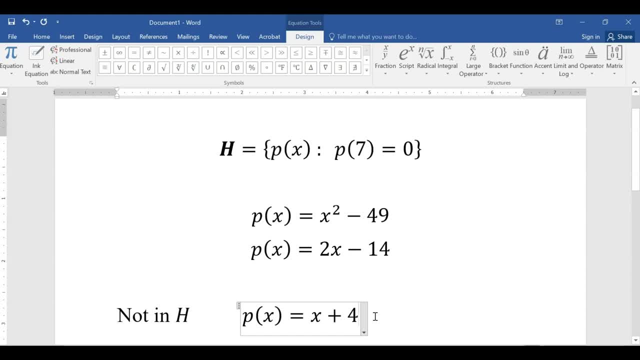 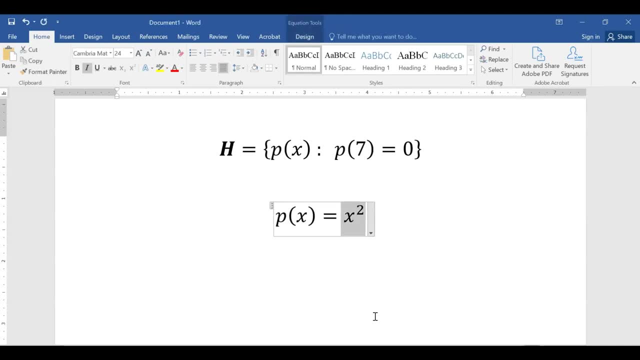 something other than zero, then it's not in H. alright, so let's think through if this set could in fact be a subspace of polynomial functions of degree three or less. so the first question is: is the zero vector in here? and I say yes, the zero vector. 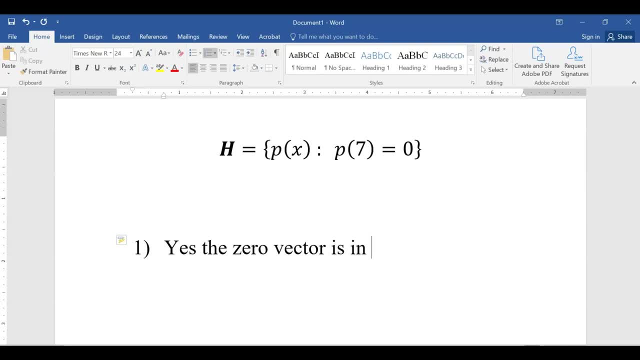 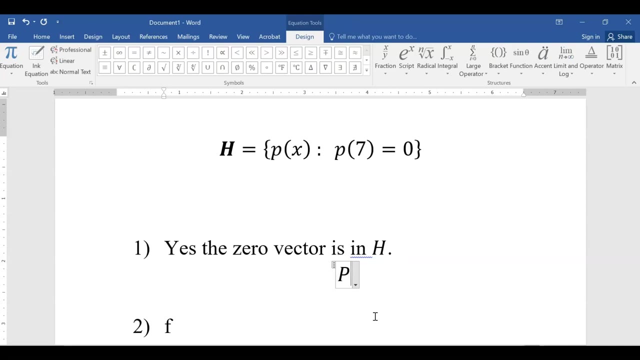 is in H, and that's pretty obvious why, if you took the polynomial function, that is the zero function. by the way, the zero polynomial is just P of X equals zero. so the zero function is that when you plug in seven into the zero polynomial, you get out of zero. so yes, 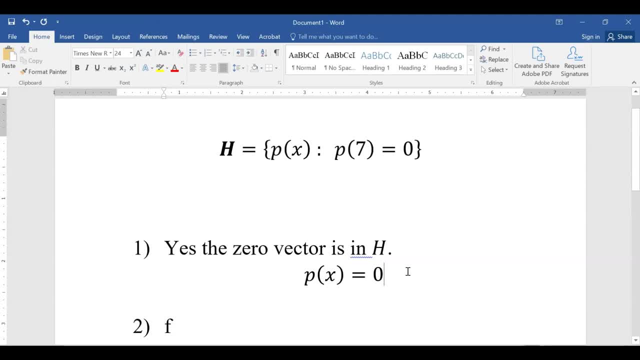 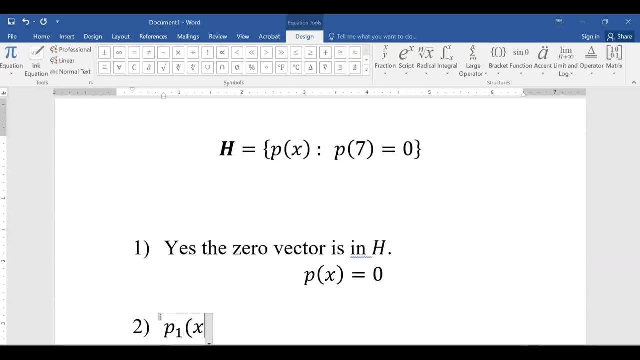 that zero vector is in H. alright, let's think about addition. so is H closed under addition? so assume I have two polynomials. we'll call them P1 and P2. so assume I have polynomials P1 and P2 which are both in my set. 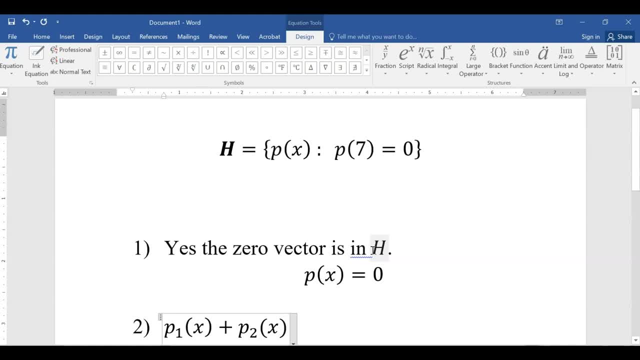 H. if you add these, you are going to get a new polynomial. now, generally, if you've seen the notation before of polynomial summations a lot of times it is something like this: right, and you want to see: is this thing in H? well, let's plug in seven. 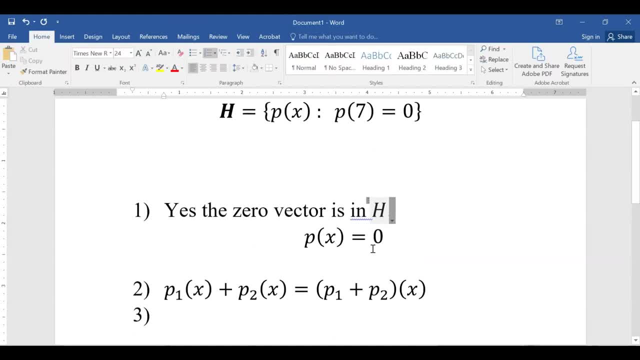 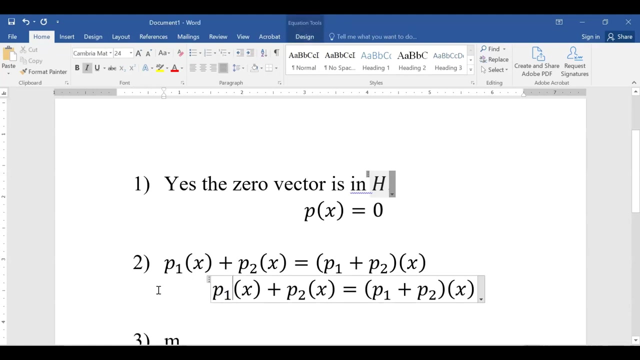 and see if we get out. excuse me, plug in seven and see if you get out of zero. so we take this sum, dang it, so plug in seven, plug in seven. so if I plug in seven into this polynomial it's the same as plugging in seven. 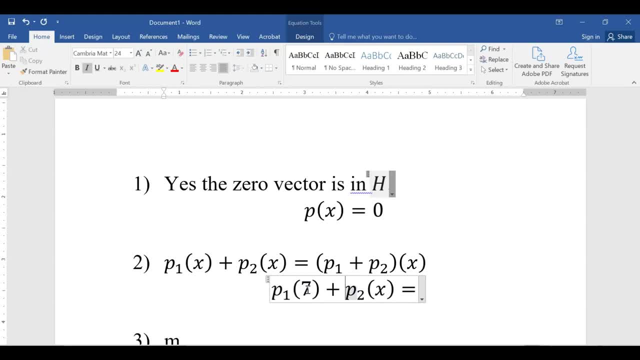 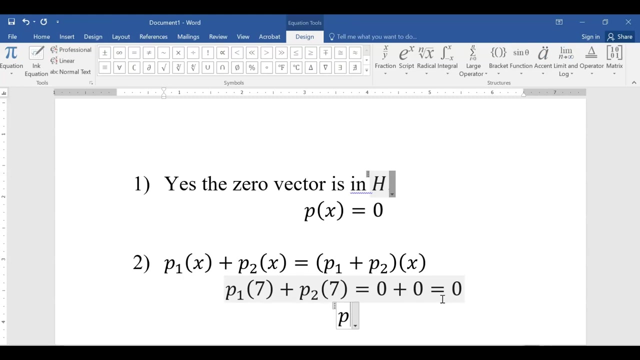 into these two polynomials individually, which gives me zero plus zero, which is zero. so yes, if you plug in seven into the sum of two polynomials in H, you will in fact get back a zero, and that means that the sum of the two polynomials is in H. 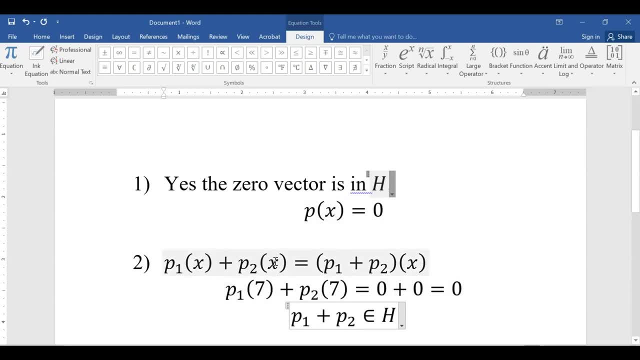 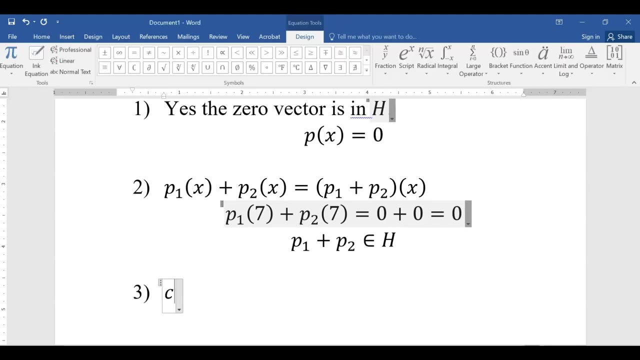 okay, so if P1 and P2 individually are, then the sum have to be in H2, because you plug in seven, you get zero. now what about scalar multiples? all you have to do is check and see. if I take a scalar times, a polynomial which I 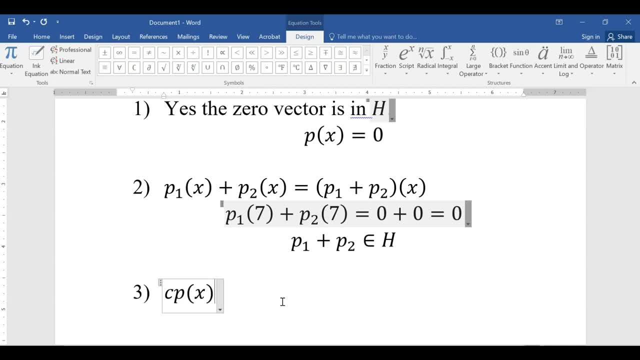 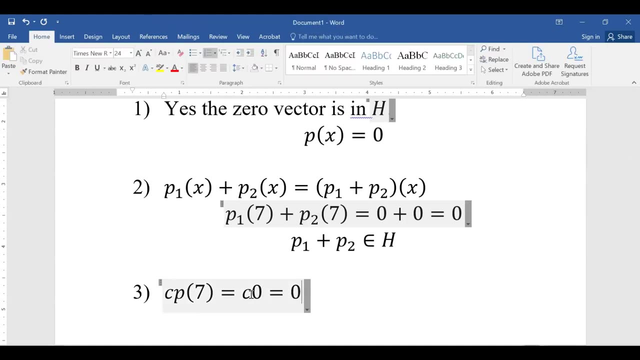 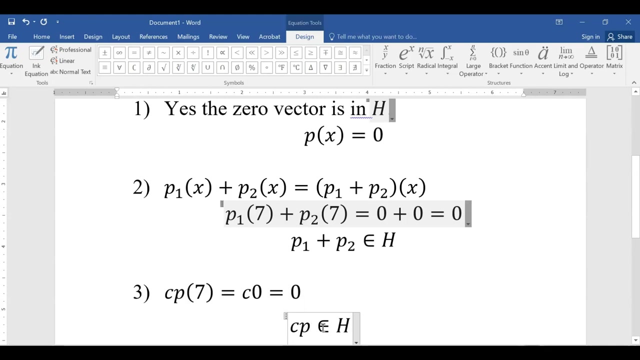 know, is already in H. what's going to happen when you plug in the number seven? well, you're going to get a scalar times polynomial. when you plug in, number seven is zero, so scalar times zero is zero, so scalar times, the polynomial is in H as well. so 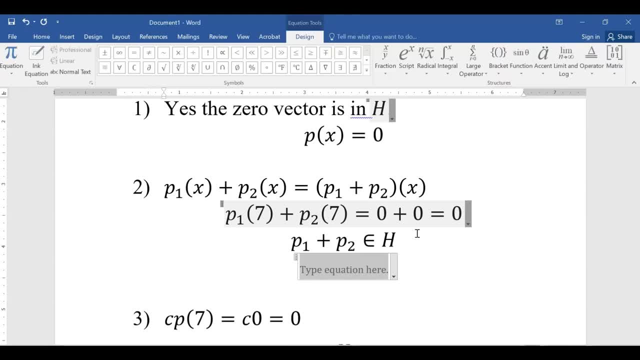 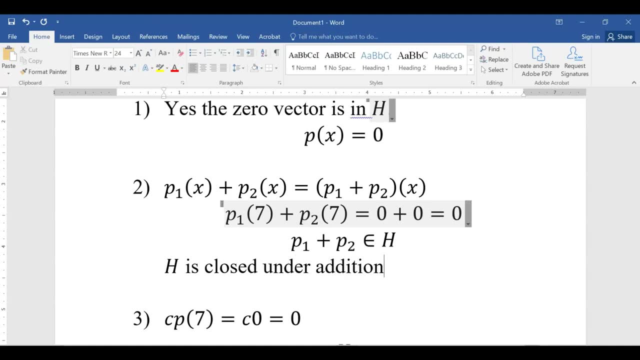 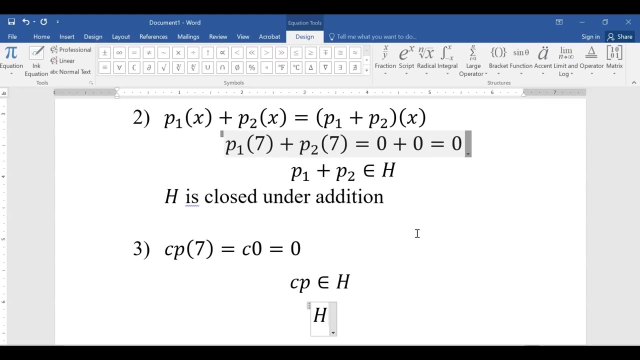 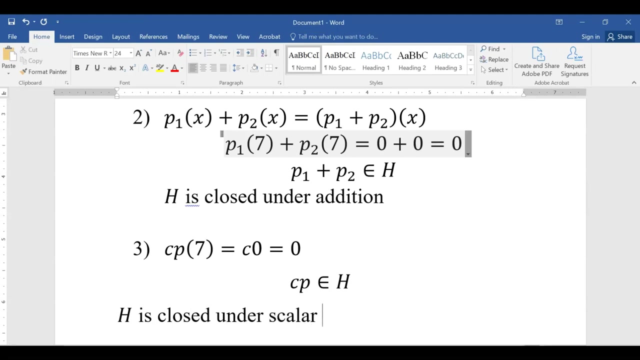 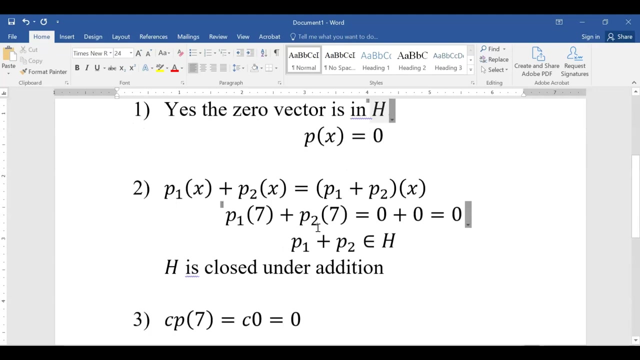 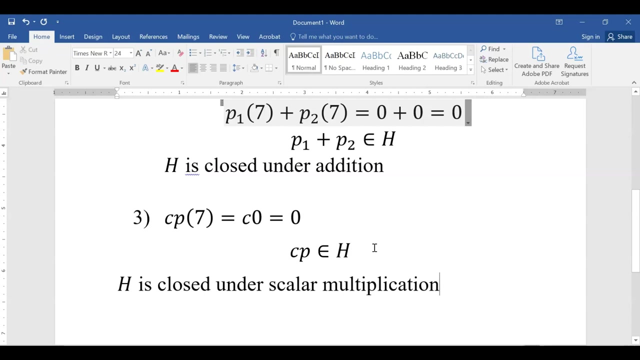 we have, H is closed under addition, H is closed under scalar multiplication and, lastly, H contains a zero vector. so because it contains all three, because it satisfies all three properties, H is a subspace, so H is a subspace, the set of all polynomials where you plug in: 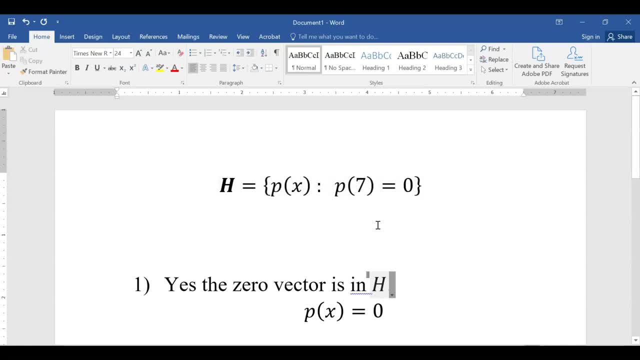 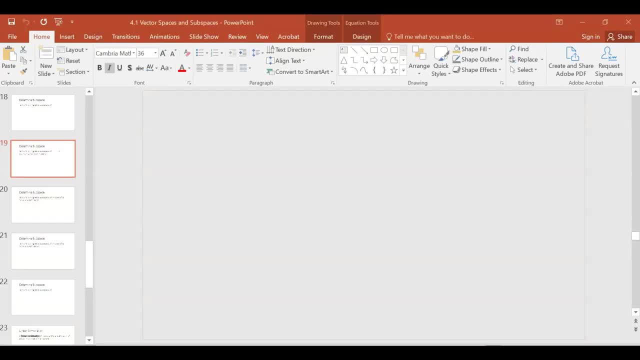 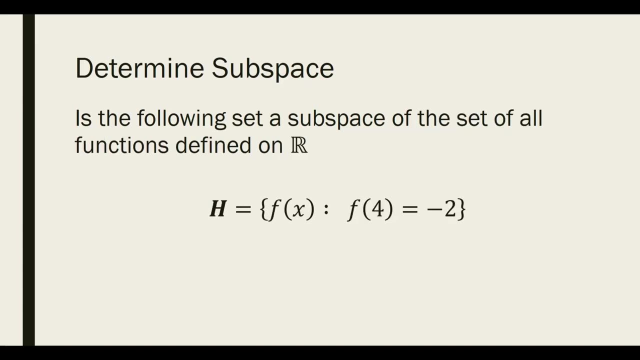 seven and you get out a zero, is in fact a subspace of all polynomials of degree three or less. okay, so there you go. I want you to determine if the following is a subspace of the set of all functions defined on R, so all functions where you plug in a. 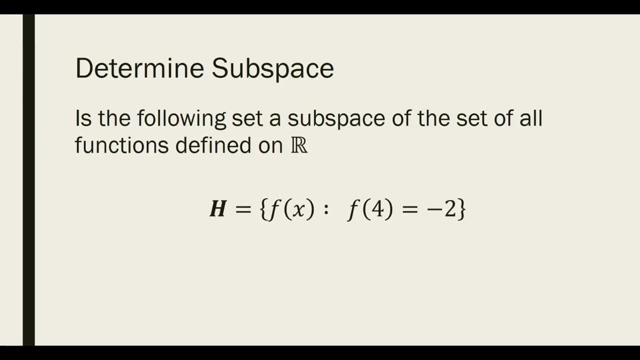 four and you get out a negative two. push pause on the video and see if you can either satisfy all three properties or show that one of these properties of subspaces doesn't hold all right. hopefully you went ahead and did that, and what you'll find is that 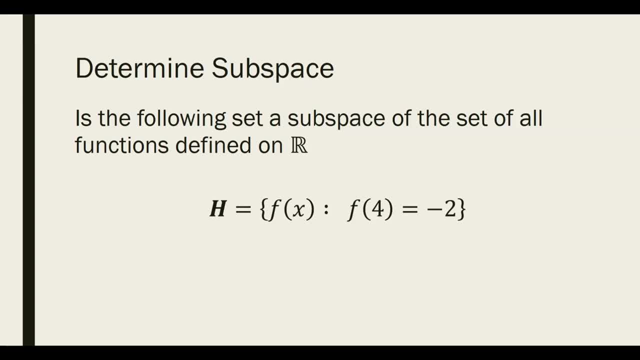 this set of functions is not a subspace. it's not a subspace because- well, for other reasons, it doesn't contain a zero vector. the zero function is f of x equals zero. no matter what you plug in, you're not going to get a negative two. 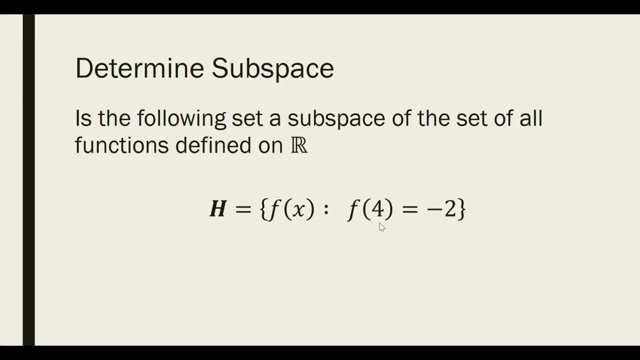 out of the zero function. so f of four would have to be zero. so this does not contain the zero function and therefore it is not a subspace. okay, how about this one? what's going to happen? the set of all functions defined on the real numbers where you plug in. 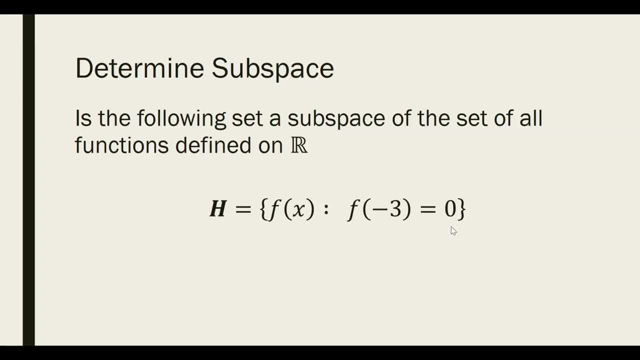 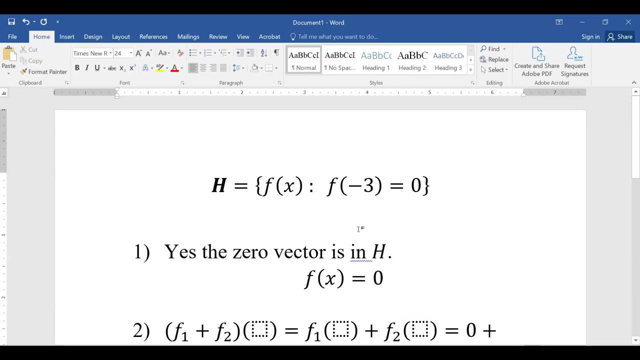 negative three and you get out a zero. I want you to try this on your own. push pause on the video. all right, so that's enough time. hopefully you did that. so we take this h and it's going to work very, very similar to what we did in. 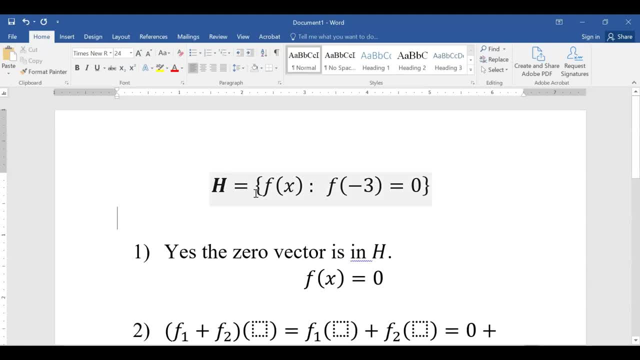 the example two slides ago. we say: set of all functions, where you plug in a negative three and you get zero. is the zero function in there? yes, because if you take the zero function and you plug in a negative three, you in fact get zero. right, the zero function is f of x equals zero. 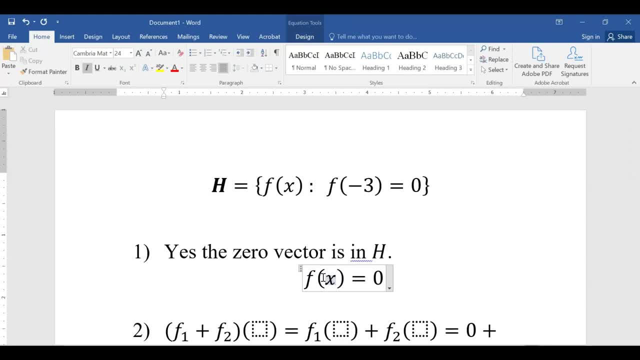 so zero function is in h, all right. what if you have two functions in h and add them? well, if you have two functions in h and add them and then plug in negative three, that's like plugging in a negative three into the first one. plug in negative three in the second one. 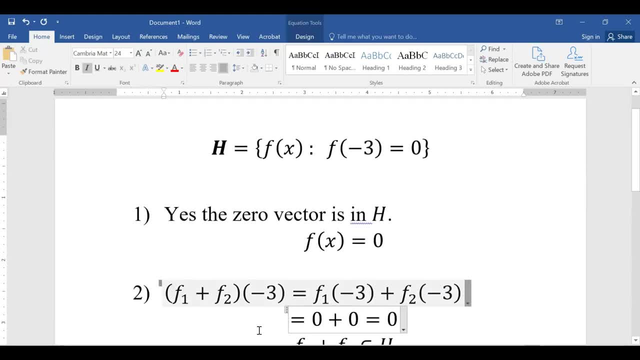 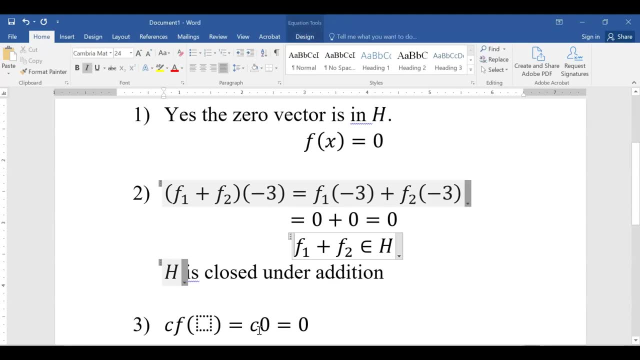 which gives you zero plus zero, which is zero. so if you have two functions in h, then the sum of those two functions is also going to be in h. so h is closed. under addition, now what about scalar multiplication? well, if i have a function in h means i plug in three. 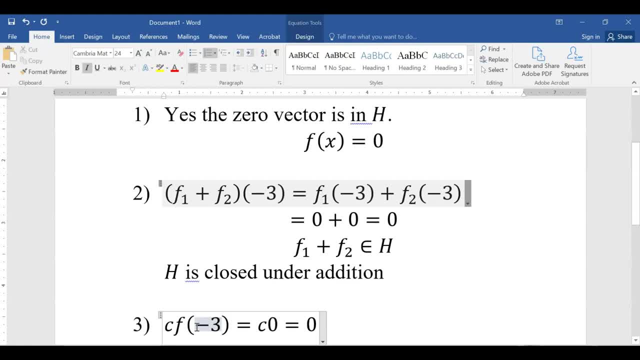 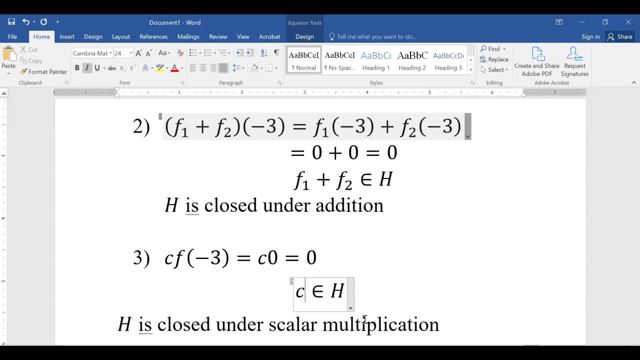 as we plug in negative three and get a zero. if i multiply that by a scalar, that's not going to change, getting out a zero. so any constant times a function in h will also be in h. so h is closed under scalar multiplication too. so we're closed under addition. 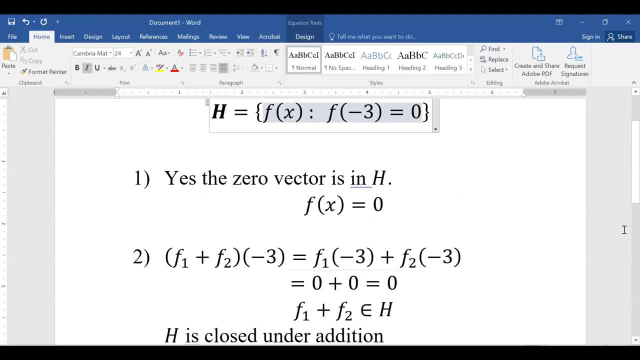 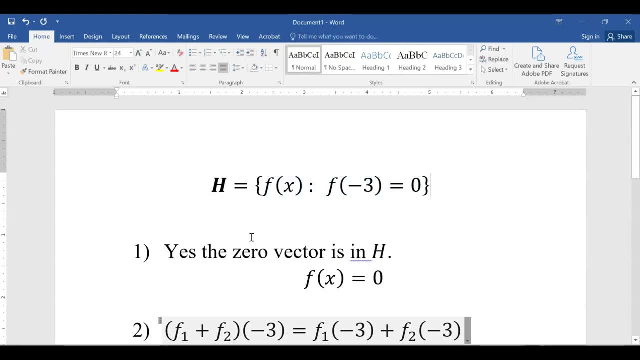 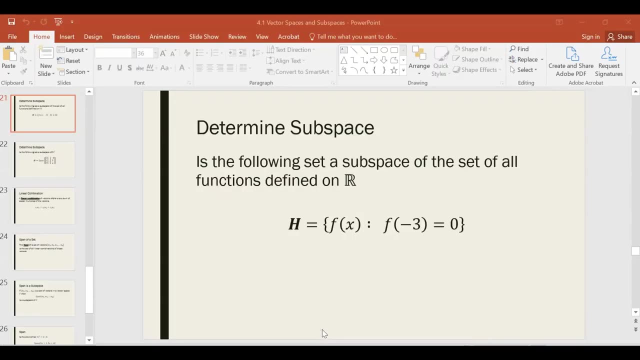 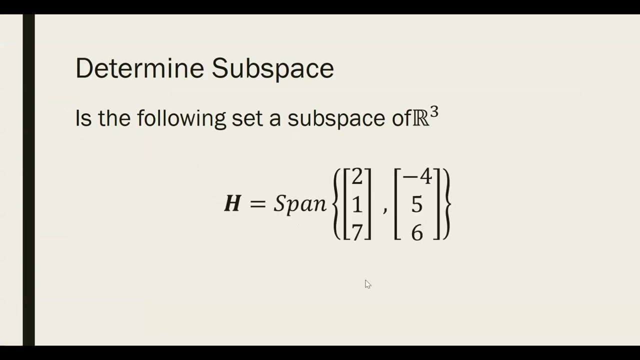 closed under scalar multiplication and contains the zero vector. therefore, h is in fact a subspace of the set of all functions defined on the real numbers. so there you go. that's what's happening now. i'm not going to go through this, in particular because i hope you remember. 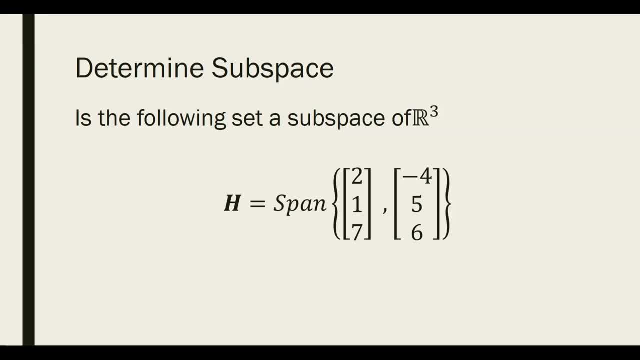 um, the idea of a span back from chapter two. remember the span was the set of all linear combinations. we showed back in chapter two that if we have the span of, for instance, two vectors, a linear combination of these two vectors, could we get the zero vector. yes, we could just make the. 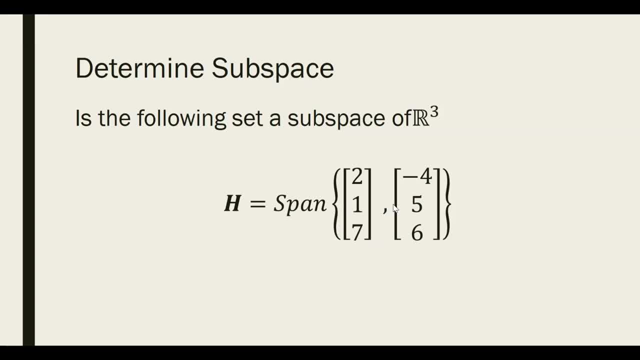 coefficient of this be zero plus the coefficient of that one be zero, and you end up with the zero vector. if you add two linear combinations, the sum is also going to be a linear combination. so the span would be closed under addition and if we did a scalar multiple. 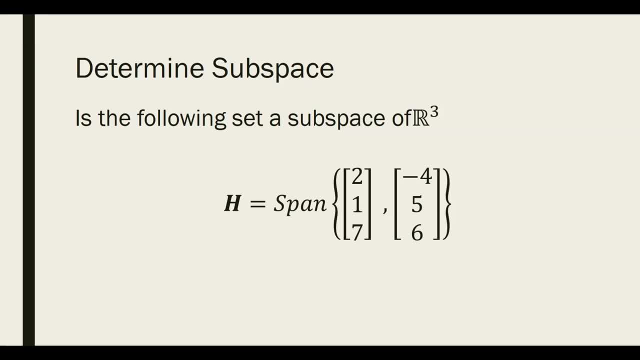 of any vector in there. it's a linear combination. if i take a scalar multiple times a linear combination, it's still a linear combination. therefore, this h, because it is the span of a couple of vectors, has to be a subspace of r3. okay, and we defined 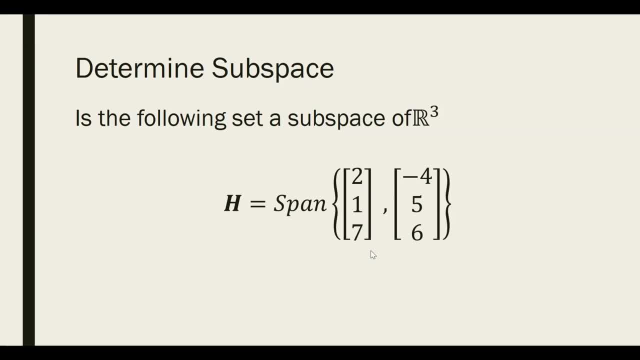 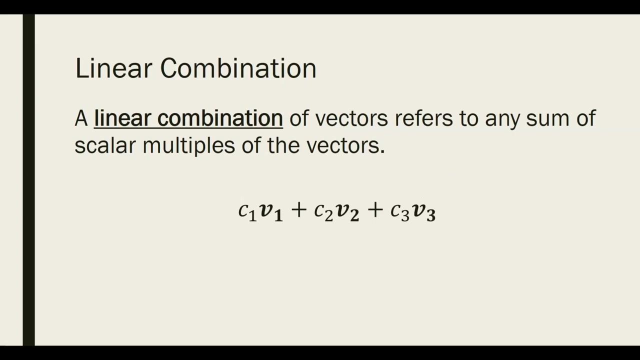 this in chapter two, this idea of linear combination and this idea of span, maybe even as far back as chapter one. but we can generalize that to not just r3 but to any vector space we want. so let's assume i have a vector space, a linear combination of vectors. 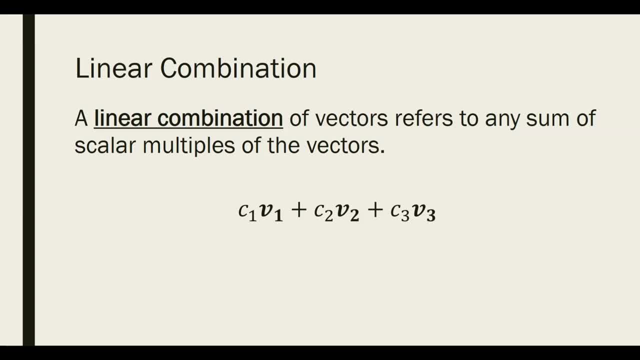 means exactly what you think it does. it means that we take scalar multiples times the vectors and then add up the result. so a linear combination is exactly the same as a linear combination of rn. but now we can do it for polynomials, now we can do it for. 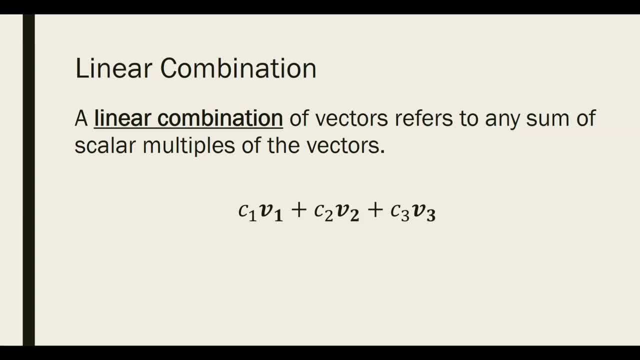 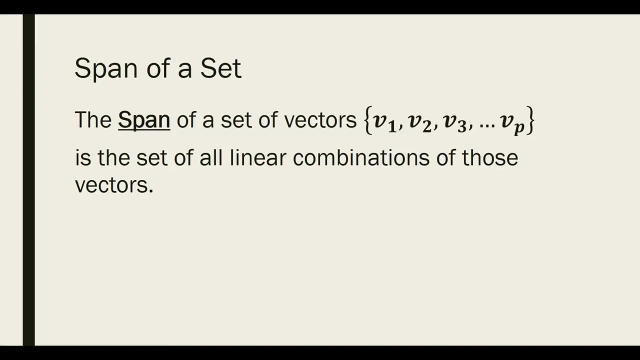 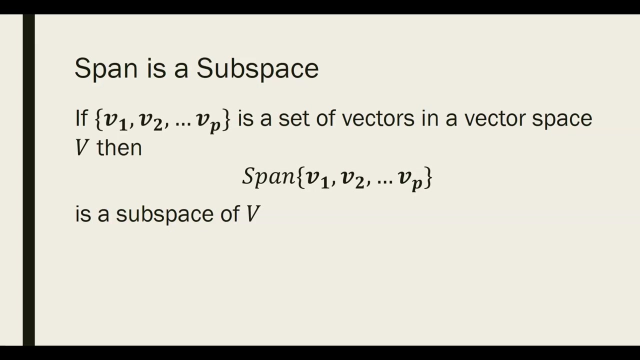 the set of all functions defined on the real line. we can do it for infinite sequences and so on and so forth. and, just like we had before, we're going to define the span of a set of vectors as the set of linear combinations of those vectors. now, 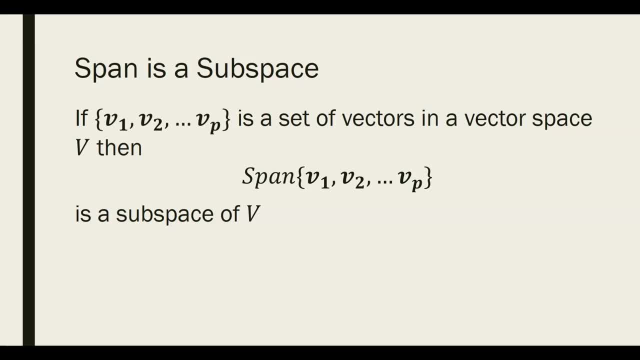 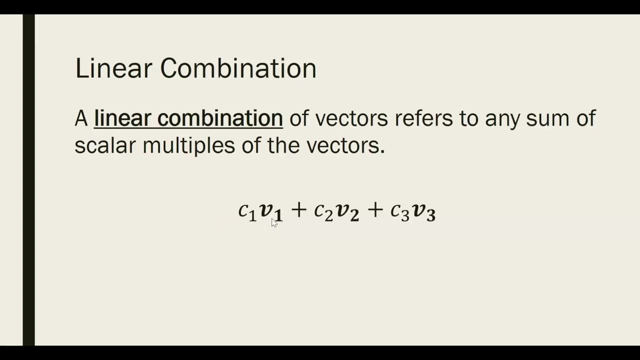 it's pretty easy to say that. it's pretty easy to show that the span of any set of vectors has to be a subspace. and the reason it has to be a subspace is because- again, think of linear combinations- there's a way to get a zero vector. 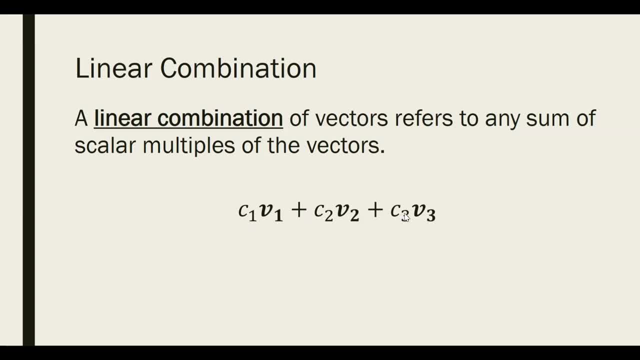 just make c1, c2 and c3 all be zero. if you add two linear combinations, then you're going to get a another vector which is a linear combination, and if you take a scalar multiple times a linear combination, you're just going to get another linear combination. 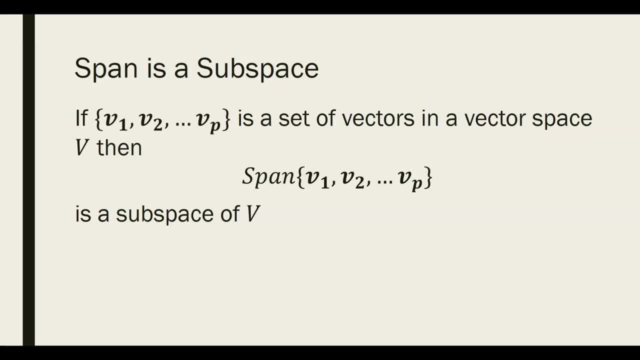 so the span has always going to have the zero vector. it's always going to be closed under addition, it's always going to be closed under scalar multiplication. therefore, spans are always subspaces of the vector space that these original vectors come out of. alright, so if these vectors came out of 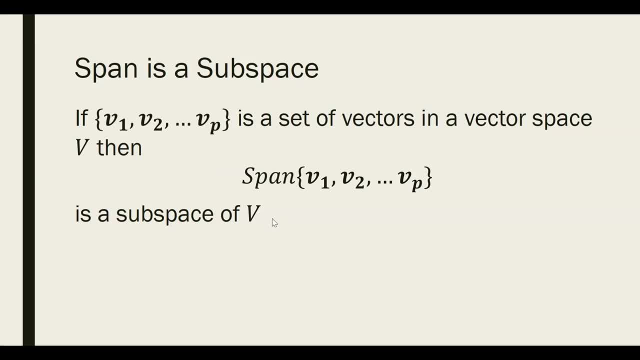 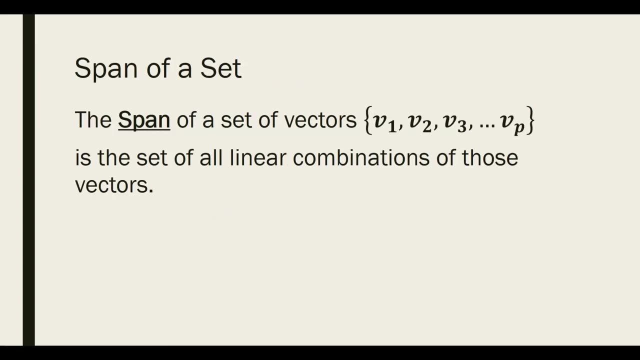 r3, the span would be a subspace of r3. if these vectors came out of r2, span would be a subspace of r2 and etc, etc. so linear combinations are the same concept we had. span is the same concept we had and we can show that the span 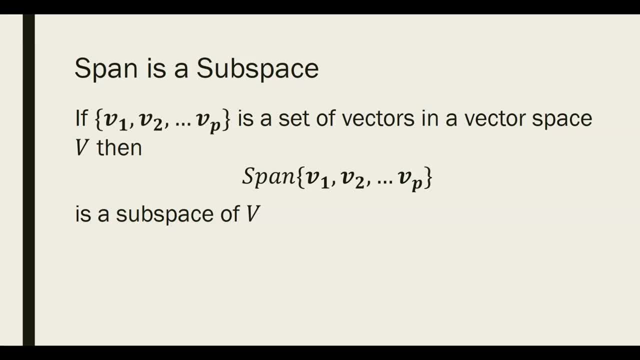 of any set of vectors is a subspace of any of the vector space they come out of. so now we know all spans are going to be subspaces and we can start asking, for instance, about the span in particular: is the polynomial 3x squared plus 2? 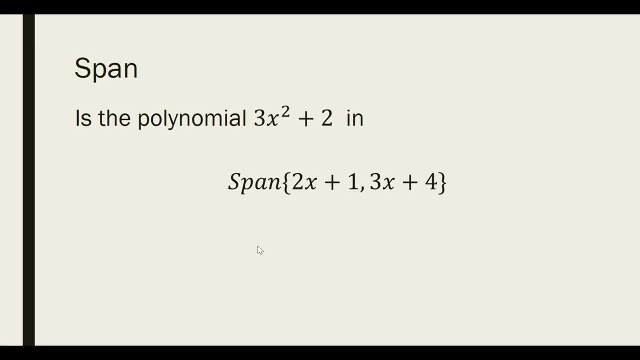 in the span of these two vectors. alright, now this is equivalent to asking: is the polynomial a linear combination of these two vectors? I want you to pause on the video and see if you can figure out if that polynomial up here is a linear combination of those two vectors. 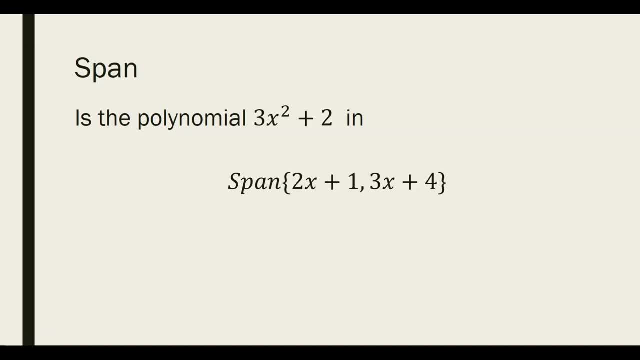 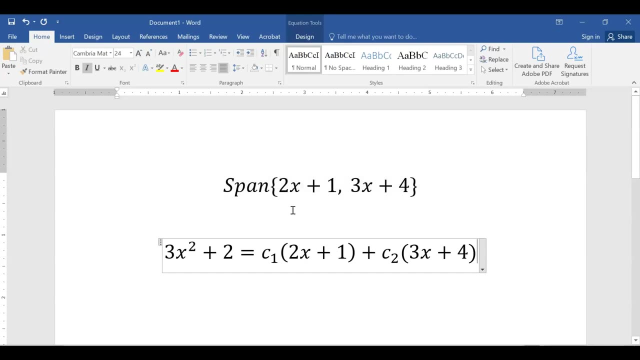 alright, so hopefully you went ahead and did that, and what I will do is I will do this. so we were talking about the span of these two linear functions. now, the fact that they are linear should be a giveaway that, in fact, this quadratic is not going to be. 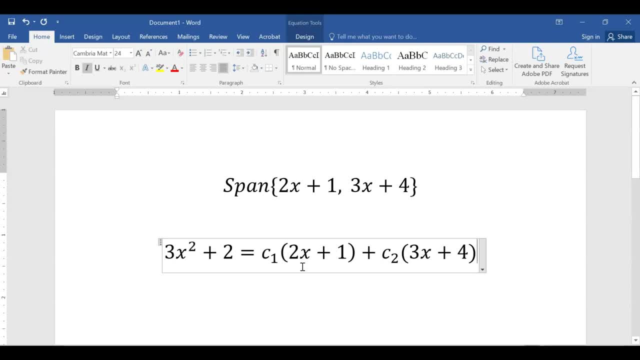 able to be written as a linear combination of these two linear functions. remember to be a linear combination. we can only have coefficients on this that are real numbers. so it's a quick argument to say that this coefficient, no matter what real number it is, when you multiply it times 2x. 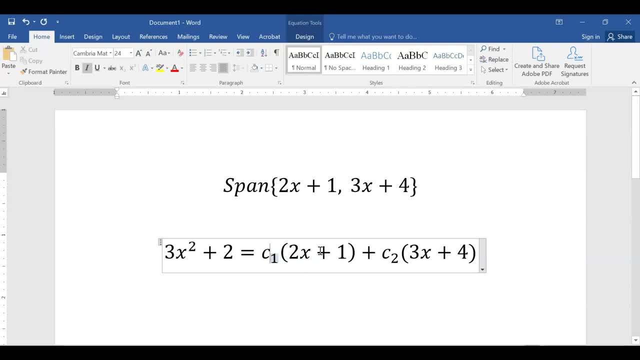 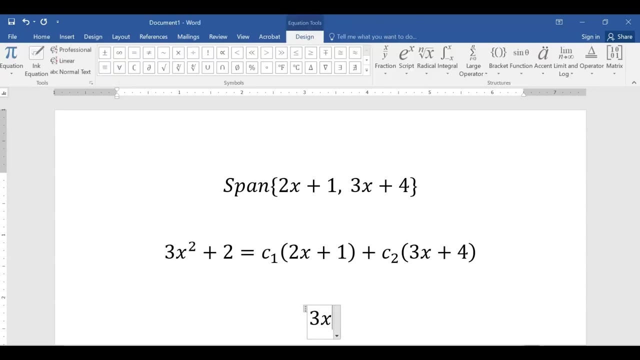 we are going to get a linear function here. in fact, let me go ahead and do that the right hand side here. so we'd have 3x squared plus 2 would have to be equal to 2 times c1 times x plus c1 plus. 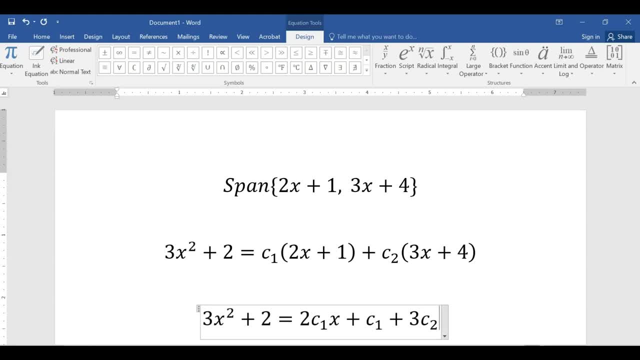 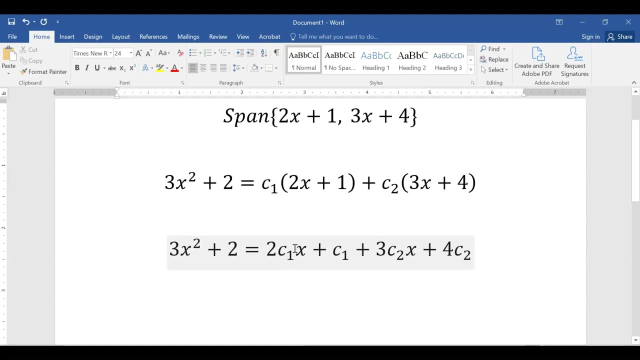 3 times c plus 2, x plus 4c, 2, and no matter what's going to happen, the right hand side is going to be a linear piece. we're going to have coefficient times x, coefficient times x, so the left hand side is quadratic. 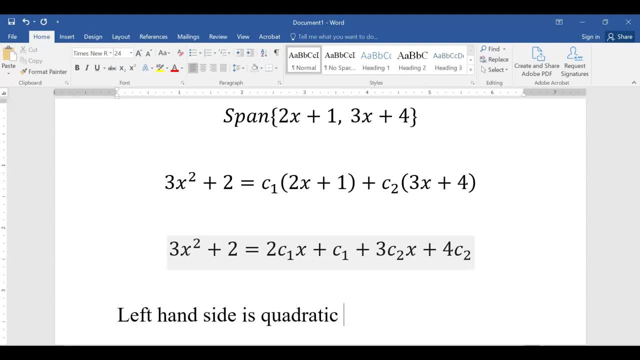 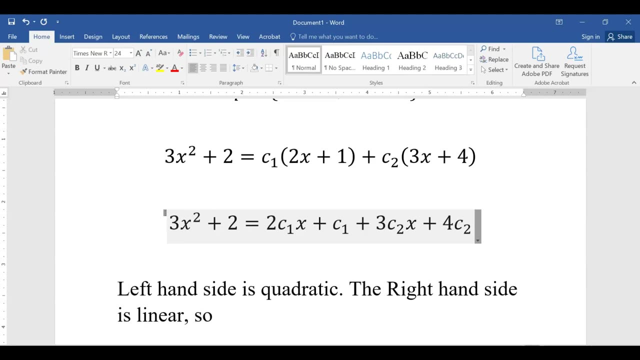 the right hand side is linear, so 3 x squared plus 2 is not a linear combination which is not in the span. ok, again, hopefully you go ahead and see that. another, I can rewrite this: when you combine like terms, you can see that more clearly. ok. 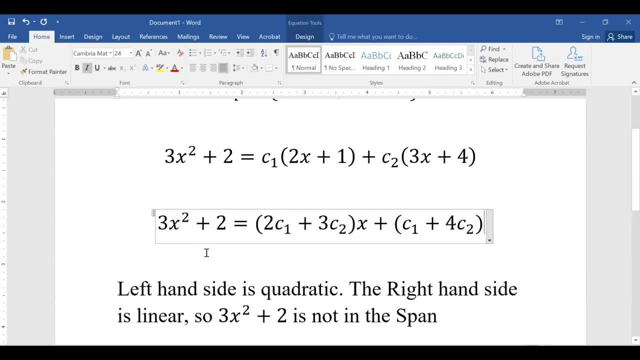 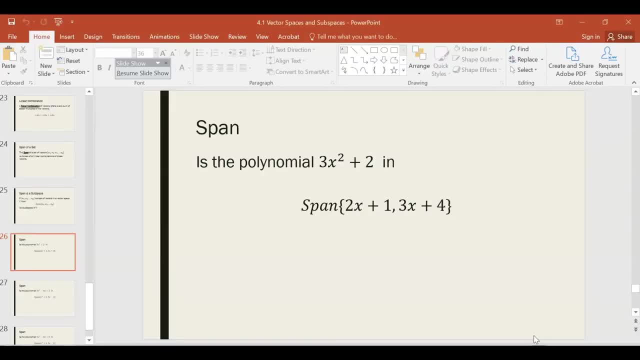 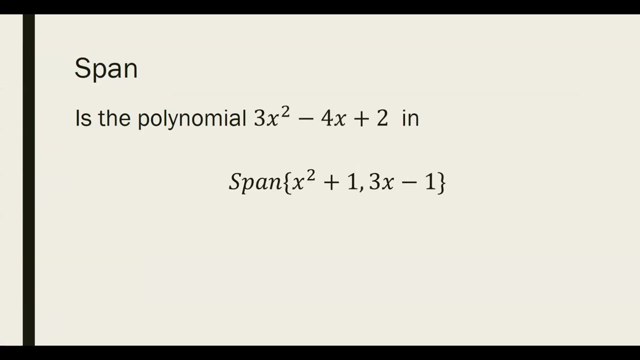 so we have a real number for an x. here we have a 3x squared, so can't in this case be in the span. I want you to go ahead and try to do this next problem: see if this polynomial can be in the span of x squared plus 1. 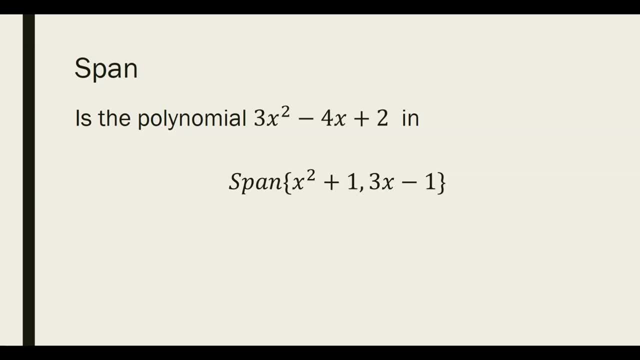 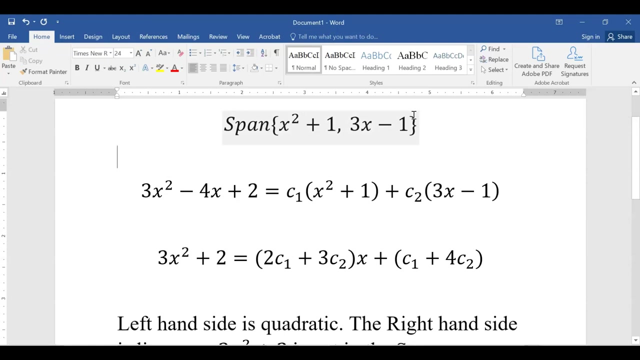 and 3x minus 1. push pause on the video and see if that can happen. alright, so we want to see if this span works. so here's what we do: we go to span of this and we try to write down my polynomial: 3x squared minus 4x plus 2. 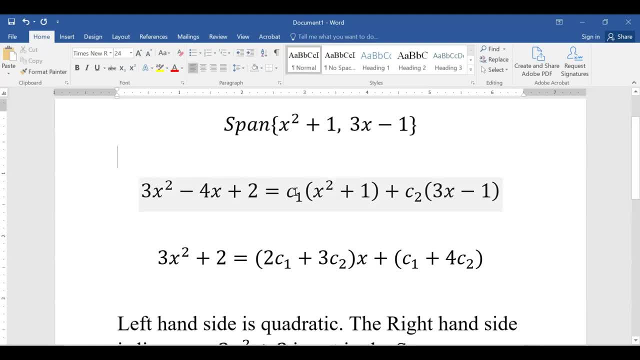 as a linear combination of these two polynomials. over here now. what I like to do is I like to multiply things out and combine like terms, so I'm going to do that. my x squared terms- the only x squared terms I have- is over here now, if I 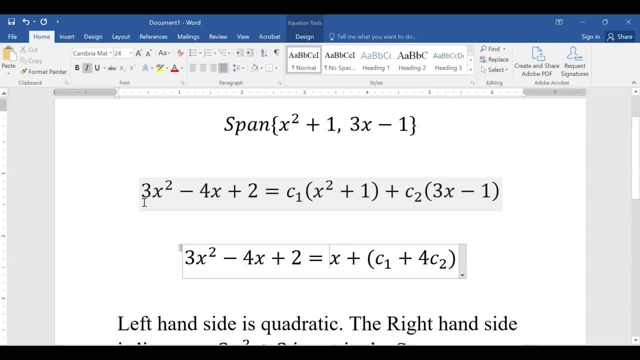 want the right hand side to match up with the left hand side. this is going to force me to have c1 equaling 3. does that make sense? we have a squared piece. maybe it will be easier to see if I do it this way. let me. 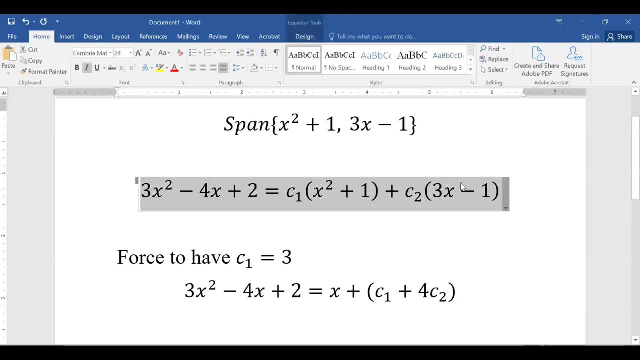 go copy and paste again. alright, so let's multiply c1. I'll distribute that out: c1 x squared plus c1 plus 3 times c2x minus c2x minus c2x, alright, and then I can combine the c1 minus c2. 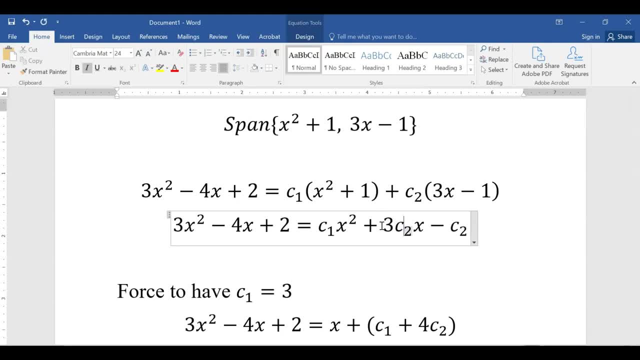 into one constant over there, alright, so notice that the coefficient of x squared on the right hand side has to be c1. the coefficient of the x squared on the left hand side has to be 3, so I have to have: c1 is equal to 3. 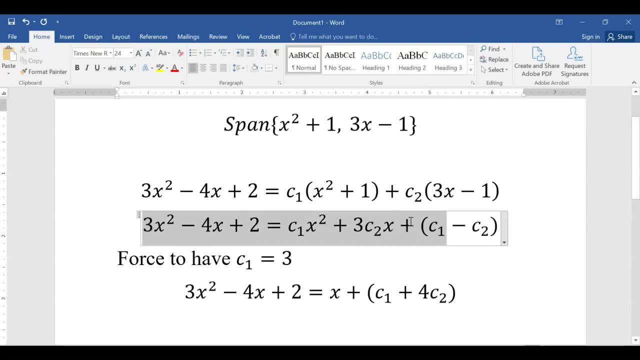 so I can rewrite this with a 3 replacing each c1. I have alright, alright, alright, alright, and if I want to, I can get rid of. by subtracting 3x squared from both sides, I can get rid of my quadratic piece, my x squared terms. 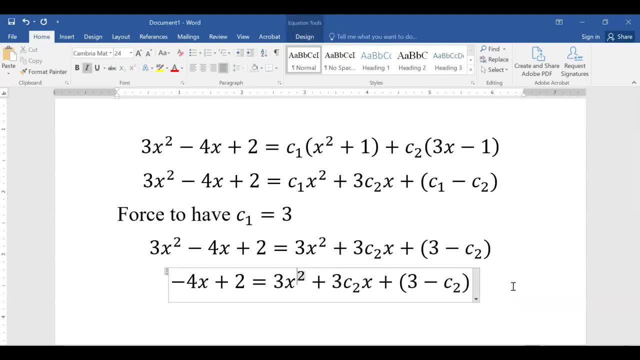 so I can subtract 3x squared. I'd get rid of it there. I could subtract 3x squared. I'd get rid of it there now. notice what's going to happen here now. notice what's going to happen here. in order: in order: in order: 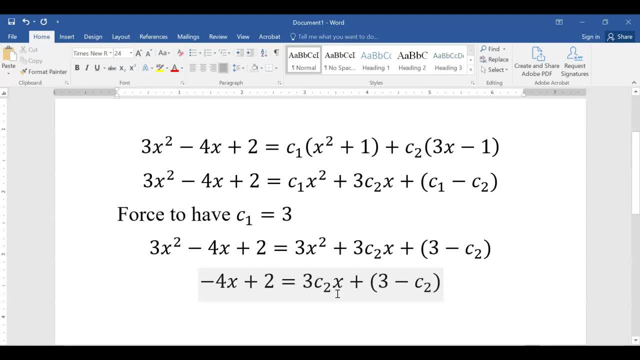 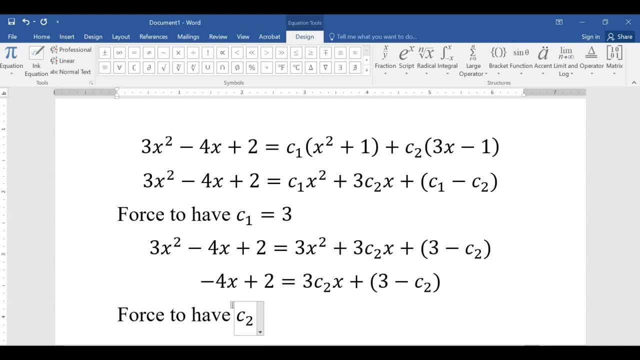 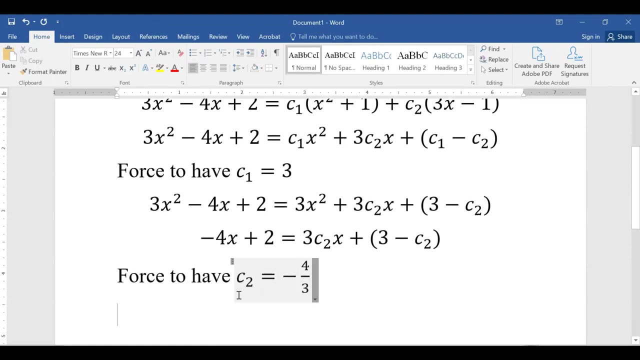 for my linear terms, my x terms, to match up. this would force me to have c2 equaling negative 4, 3rds. hopefully that makes sense that in order for you to multiply times a 3 and get a negative 4, you're going to have to have negative 4 3rds. 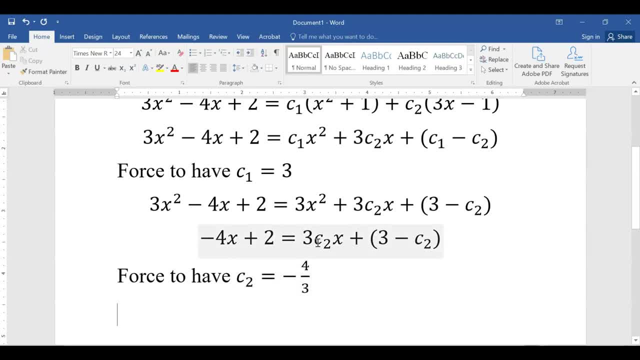 you're going to have to have negative 4- 3rds if I'd plug in negative 4 3rds into there. let's go ahead and do that. let's go ahead and do that. so plug in a negative 4- 3rds. 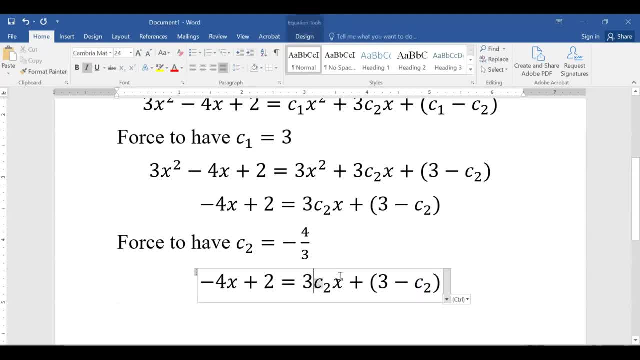 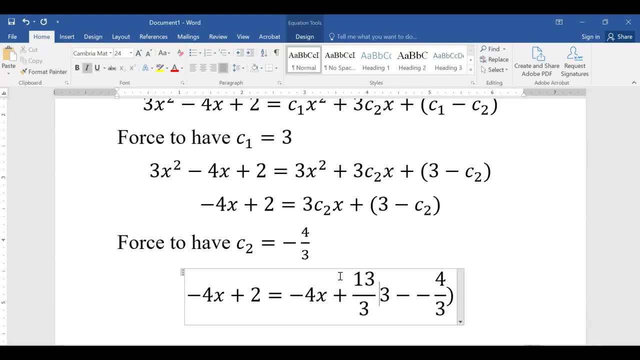 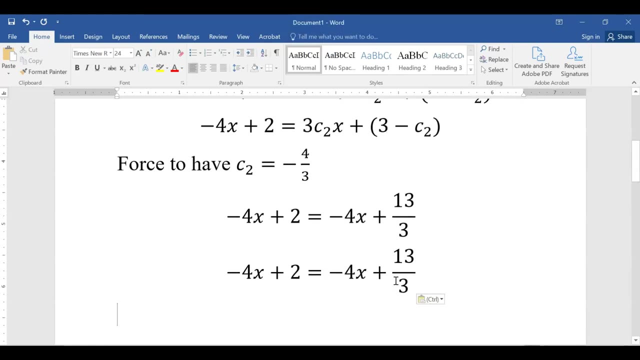 By the way, that would be 13: 3rds as a fraction, And if you added 4x to both sides- Add 4x to the right hand side And add 4x to the left hand side- What you see is you get a false statement. 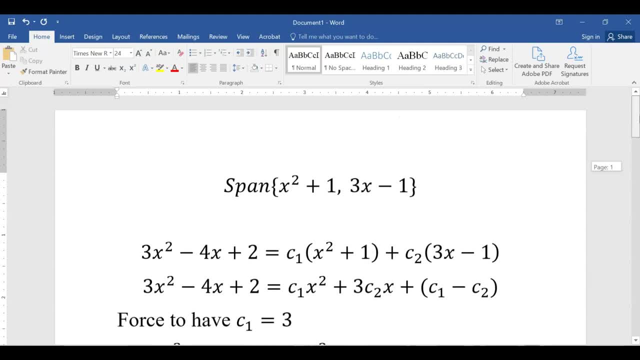 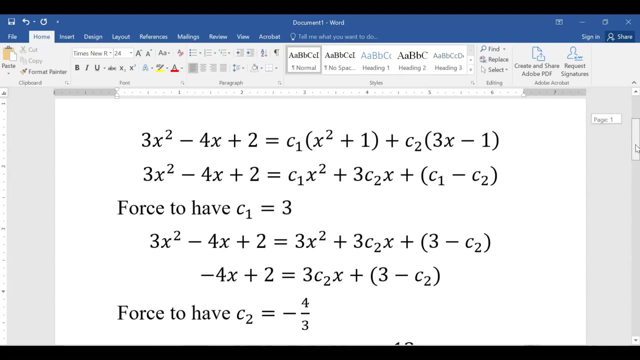 So what I'm trying to get at is that there is no linear. so therefore, no matter what you did in order to make this equal, in order for us to get a linear combination that actually works out, We came with a false statement. 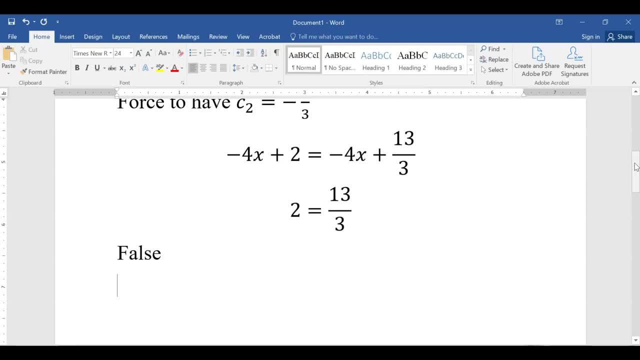 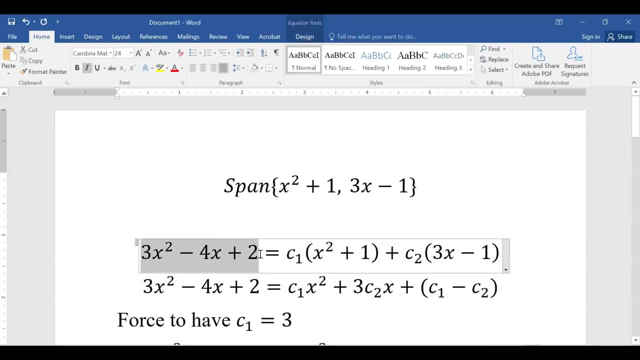 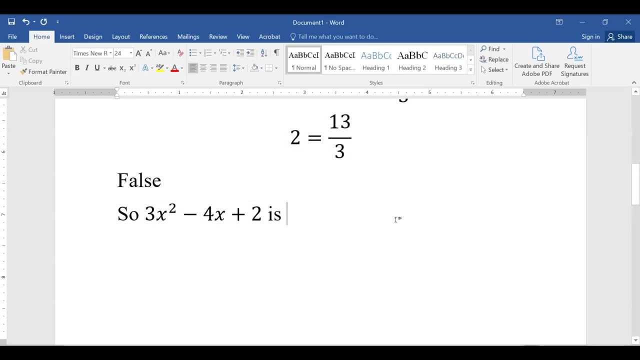 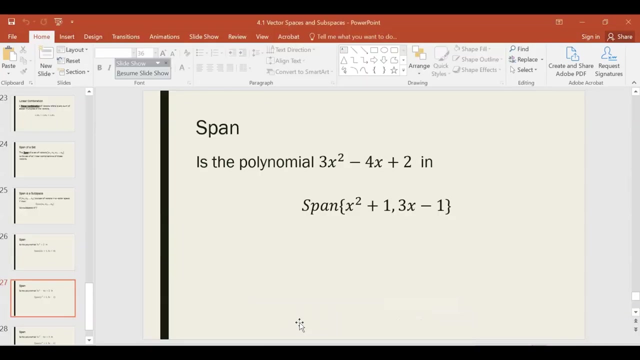 Therefore, that original function we started with this- 3x squared minus 4x plus 2, cannot be in the span because it cannot be written as a linear combination. Okay Again, hopefully you went ahead and did that. Now let's do this just one more time. 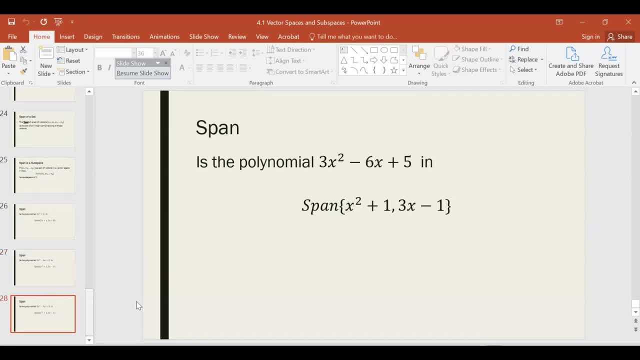 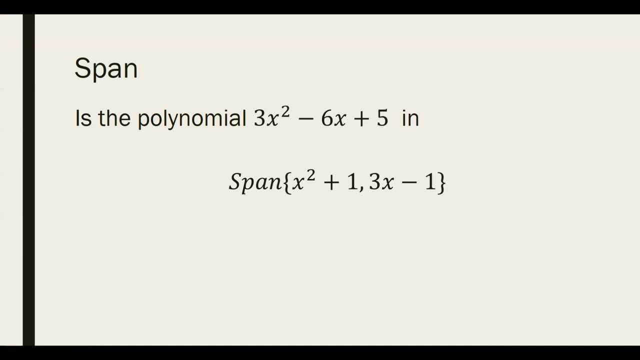 And I want you to determine There we go. If this polynomial 3x squared minus 4x, What is the final constant? minus 6x plus 5 can be in the span of those two functions. I had Push pause on the video and see how this turns out. 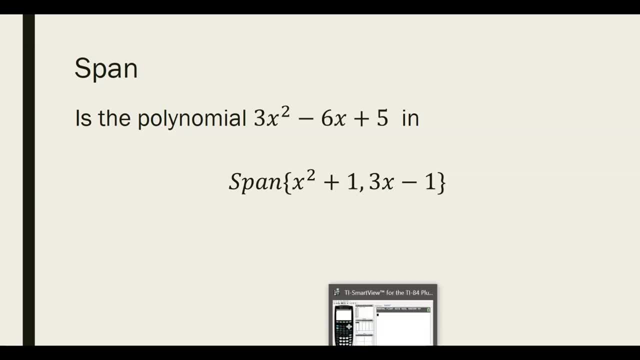 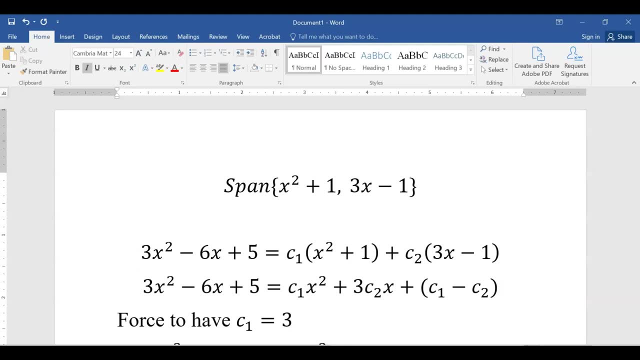 Alright, hopefully you did that. Alright, so hopefully again you went ahead and did that. So we have our two polynomials, x squared plus 1, 3x minus 1.. We're looking to see if a linear combination of those two can add up. 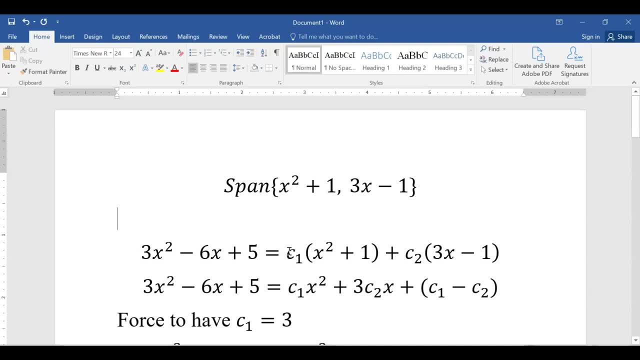 to 3x squared minus 6x plus 5.. So I just set these two things equal, the linear combination equaling 3x squared minus 6x plus 5, and hopefully I can solve for c1 and c2.. 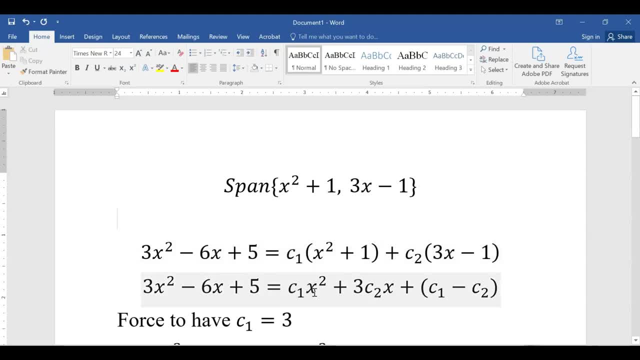 Now if we distribute c1 times x squared, c1 times 1,, c2 times 3x, c2 times negative 1, what you'll see- I'll start with the x squared terms, Again: 3x squared. the only x squared I have on the right is: 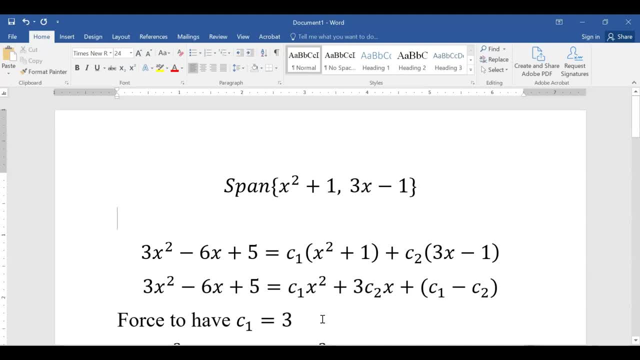 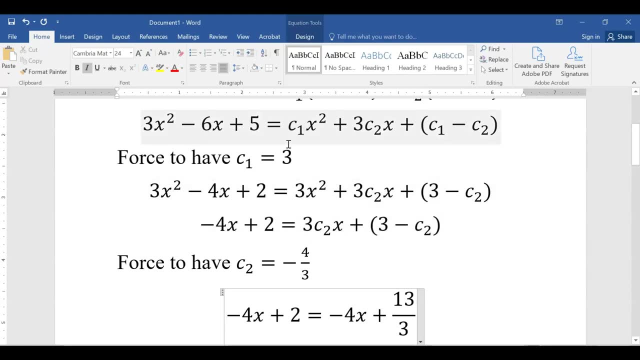 c1 times x squared, So that forces my c1 to be 3.. If I do that, c1 is 3, plug that in. oops minus 6x. I haven't changed it from the last problem. If I plug that in. 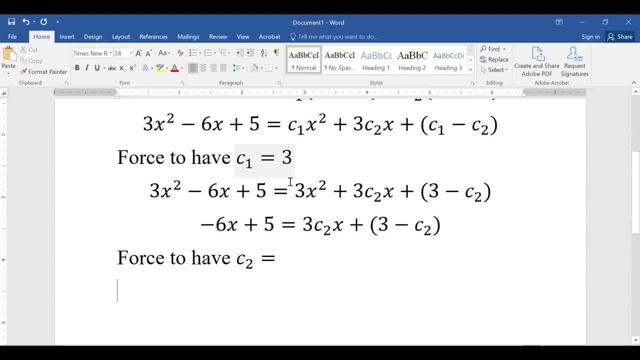 I'm sorry, I lost the coordinate almost there. My problem ends here. So subtract 3x squared from both sides, get negative. 6x plus 5 equals 3c2x plus 3 times negative c2.. Now, in order for negative 6 to be the coefficient of x, 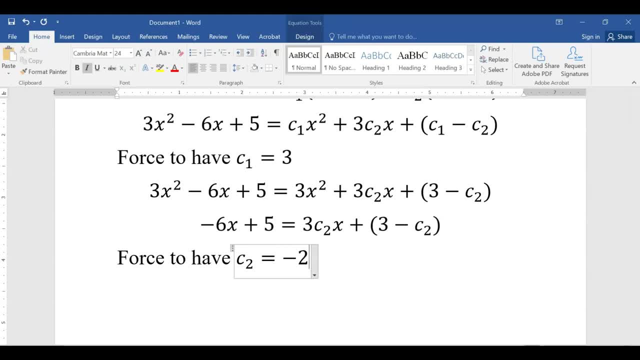 of x, c2 would have to be a negative 2,. all right, If c2 is negative 2, negative 2 times 3 becomes a negative 6.. 3 minus negative 2, that all becomes a 5..